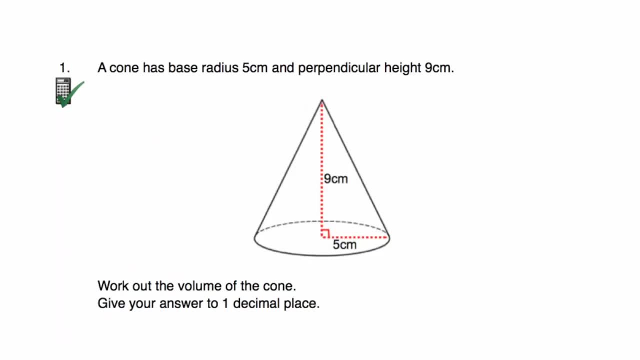 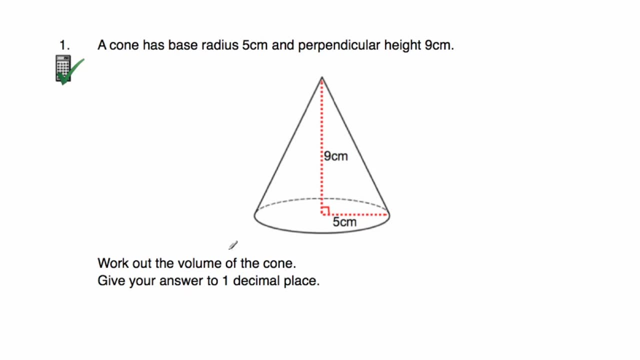 So let's get started. Question number one. Question number one says a cone has got a base radius 5 centimeters and a perpendicular height of 9 centimeters. Work out the volume of the cone. Give your answer to one decimal place. 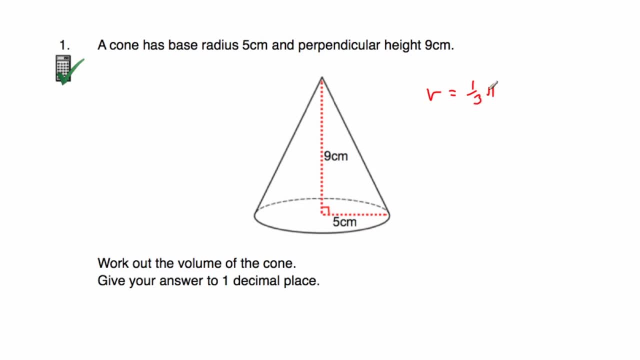 Now the volume of a cone is equal to a third pi r squared h. In other words, we're going to do a third multiplied by pi, multiplied by the radius squared, multiplied by the perpendicular height. So we know what the radius is. The radius is 5, and we know what the height is, the h, the perpendicular height. 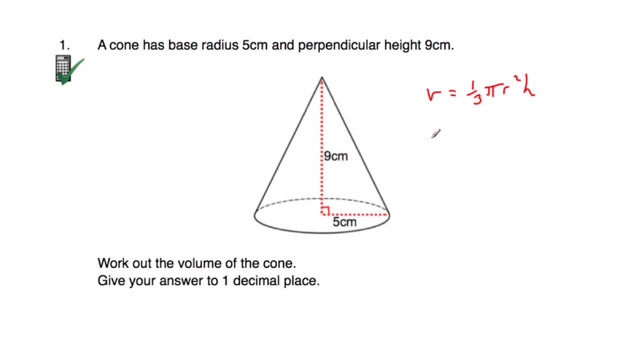 That's 9 centimeters. So let's substitute those values into the formula. So the volume is equal to a third multiplied by pi times the radius, which is 5 squared multiplied by the height, 9.. So we've substituted in r: The radius is equal to 5 and the height is equal to 9.. 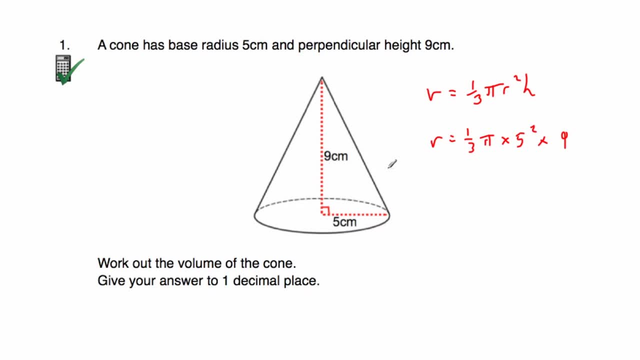 So we've substituted those in. Now we just need to work this out. Now it's a calculator question. Now, at this point we could just have to do a calculator: a third multiplied by pi, multiplied by 5 squared and multiplied by 9.. And when we do that, we get the answer: 75 pi. 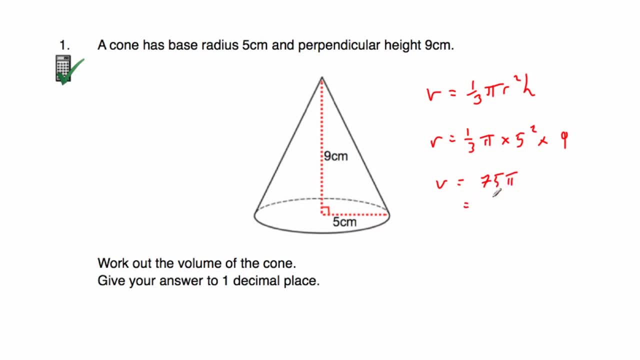 But this question wants our answer to one decimal place. So let's convert that into a decimal, So let's change that to a decimal and we get the answer 235.61945.. So we've got 4, 9 and so on. centimeters cubed. 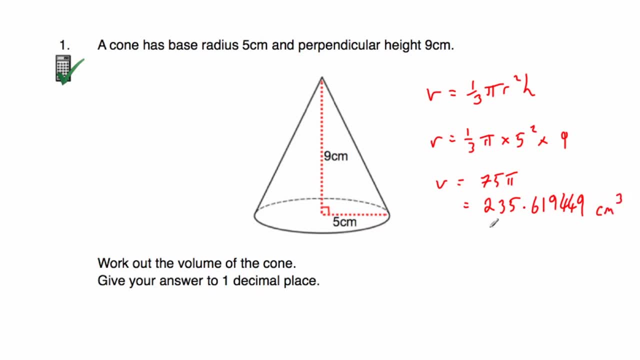 Make sure, because it's the volume. we've got our unit centimeters cubed. Now we want to round this to one decimal place. So the answer to one decimal place would be 235 point. Now we've got 6 ones, so it's just going to be 0.6.. So the answer is 235.6 centimeters cubed. 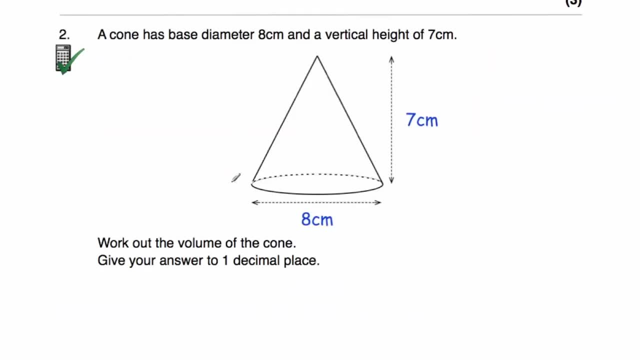 And that's it. Okay, let's have a look at question number two. So question number two says a cone has got a base diameter of 8 centimeters and a vertical height of 7 centimeters. Work out the volume of the cone and give your answer to one decimal place. 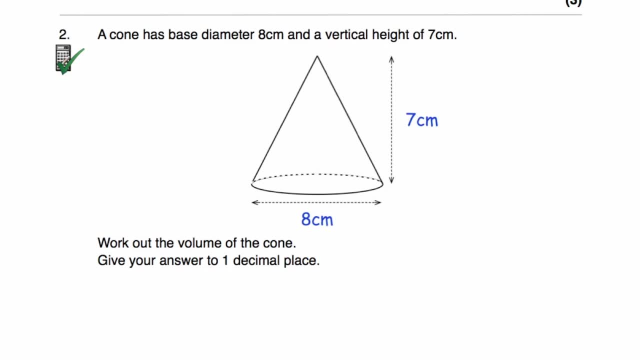 So we need to find the volume of this cone and we need to give our answer to 1.. And again, it's a calculator question. So the formula for finding the volume of a cone is: the volume is equal to a third pi r squared h. 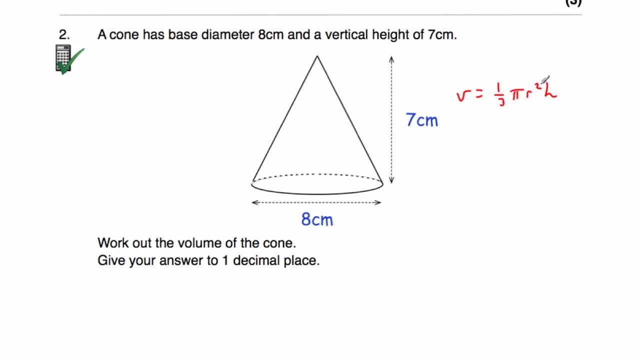 In other words, a third multiplied by pi, multiplied by the radius squared, multiplied by the height or the perpendicular height. So then the volume would be equal to a third multiplied by pi, multiplied by the radius squared. Now, if we look at this circle, it's got a diameter of 8 centimeters. 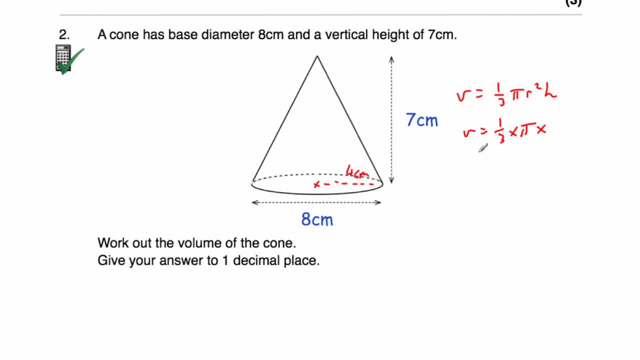 That means the radius of the base would be equal to 4 centimeters halfway across. So multiply by 4 squared multiplied by the height. And the height is 7 centimeters, so multiply by 7.. So when we type in our calculator, a third multiplied by pi, multiplied by 4 squared times 7,. 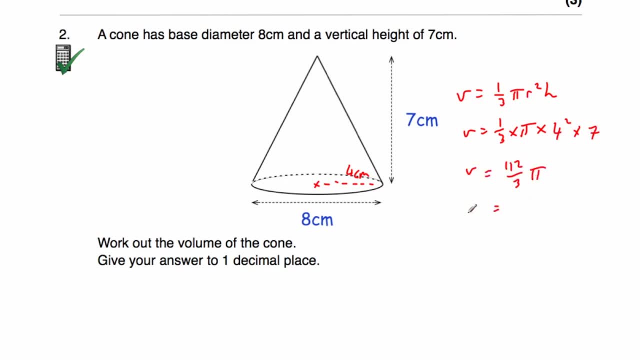 we get an answer of 112 over 3 pi, Or as a decimal number, the volume is equal to. if we change that to a decimal, 117.2861257 centimeters cubed. Now we want to give our answer to one decimal place, so our answer would be: volume is equal to. 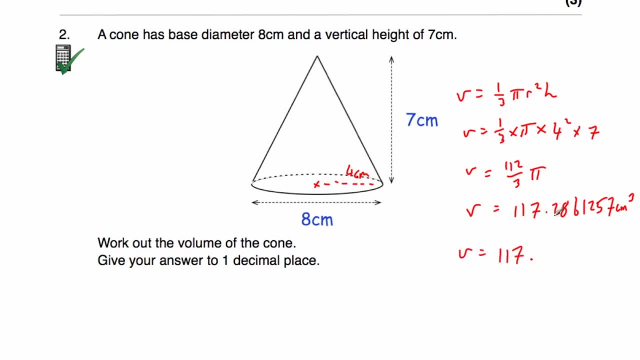 we want to round this to one decimal place, so it would be 117 point and we've got 2 eighths, so it would be 0.3 centimeters cubed. So the volume of that cone is 117.3 centimeters cubed. 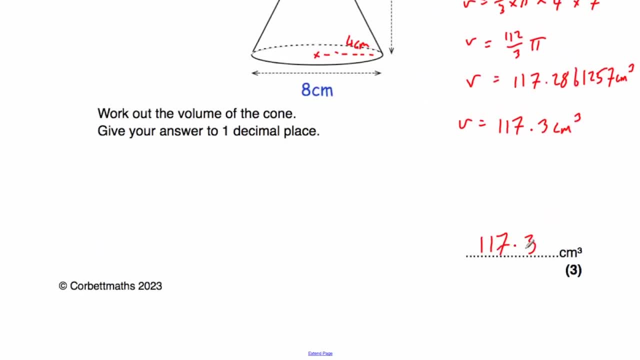 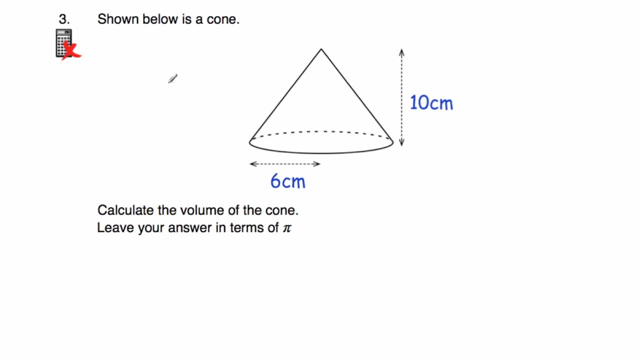 And let's just write that in the answer section. So 117.3 centimeters cubed. Okay, let's look at our next question. Okay, let's have a look at question number three. So question number three is a non-calculator question, so I've just put down my calculator. 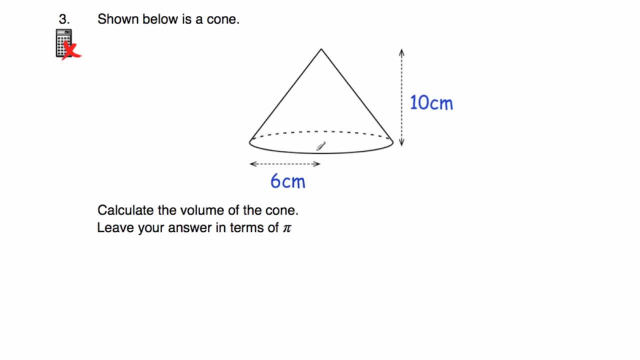 And we've got shown below is a cone. so we've got this cone and it's got a radius of 6 centimeters and a height, a perpendicular height, of 10 centimeters, the height straight up and down. And we've been asked to calculate the volume off the cone and we've to leave our answer in terms of pi. 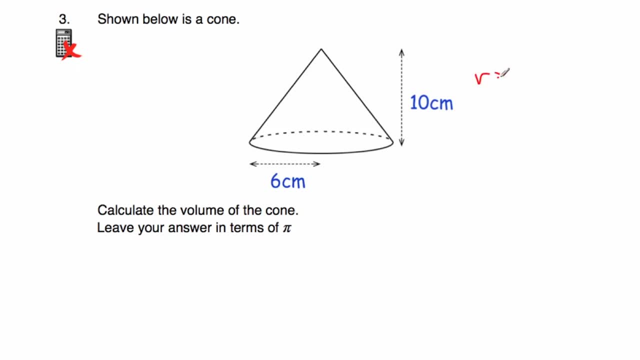 So let's write down the formula for finding the volume For cone. the volume of a cone is equal to 1, 3rd pi r squared h. Now we know the radius is 6 and the height is equal to 10, so let's substitute those into the formula. 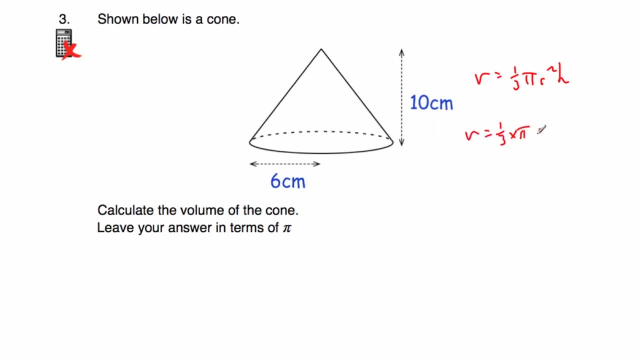 So the volume is equal to 1, 3rd, multiplied by pi, multiplied by the radius. Now the radius here is 6, so 6 squared, multiplied by the height of the cone, which is 10.. Now we need to work this out without a calculator, so let's remember our order of operations. 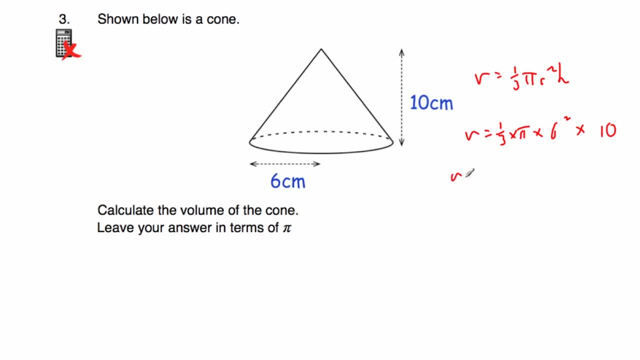 So we need to square first of all. so 6 squared is 36, so the volume is equal to 1, 3rd multiplied by pi, multiplied by 36, multiplied by 10.. So now we've got the volume is equal to 1, 3rd times pi, times 36 times 10.. 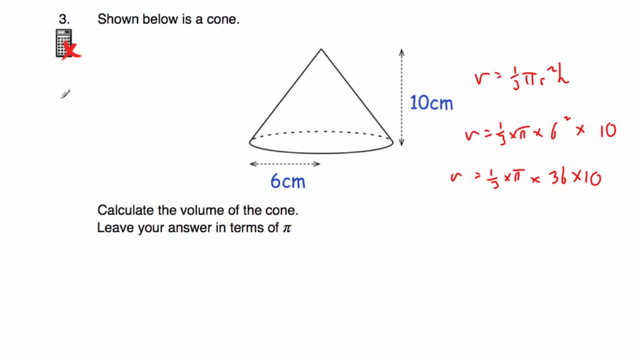 So here we're multiplying these together and remember, if we had four things and we're times them together, for instance, 2 times 5 times 10 times 4, it doesn't matter what already you multiply these in, You could do: 2 times 5 is equal to 10 times 10 is equal to 100 times 4 is equal to 400,. 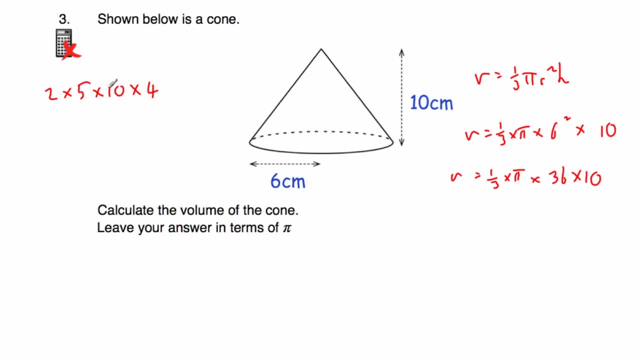 so 400 is the answer. so you could do it that way. You could do it another way. You could do: 5 times 10 is equal to 50, and then times by 2 is 100, and then times 4 is 400, and so on. 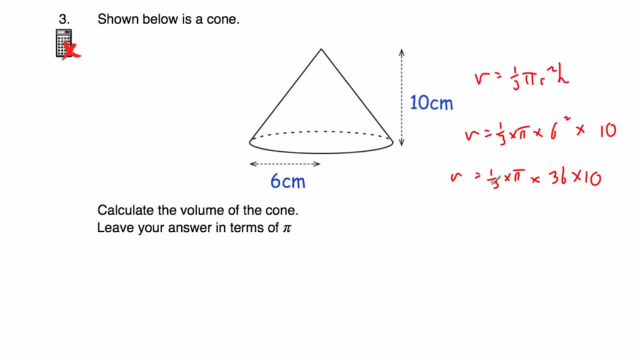 So it doesn't matter what What you multiply things in. So here we have got 1 3rd times pi times 36 times 10.. So I could do: 36 times 10 is 360, and then multiply that by 1, 3rd, which means 1 3rd of it and 1 3rd of. 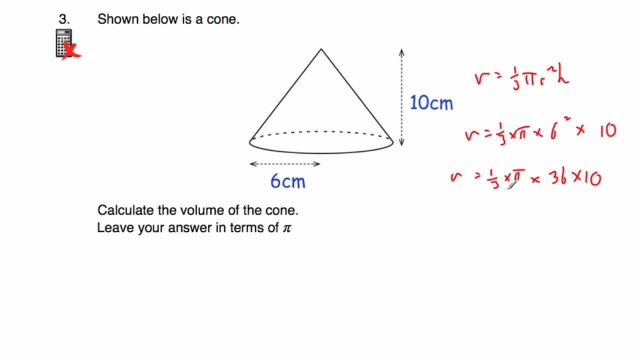 360 would be 120, and then we've got pi, so that should be 120 pi. That's one way to do it. Another way to do it is: here: I've got 1 3rd times 36, and 1 3rd times 36 is 1 3rd of 36, which is 12.. 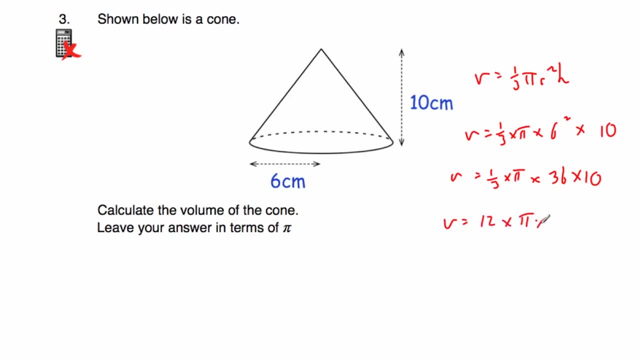 So I can write 12 and then we've got times pi and then we've got times 10.. Now I'm going to do 12 times 10, and 12 times 10 is equal to 120, and we've still got our times pi and 120 times pi. 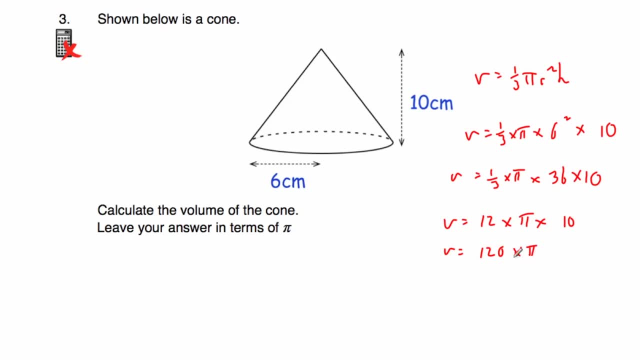 We just put them together, so the volume would be 120 pi, and remember our units- centimetres cubed, and that's it. So the volume of the cone is 120 pi centimetres cubed, and that's it. Okay, let's look at our next question. 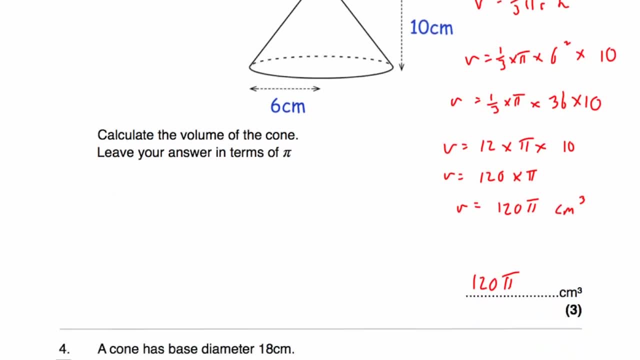 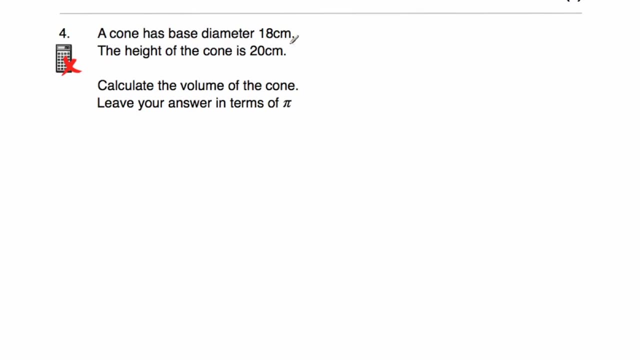 Question number four. So question number four, it's a non calculator question. So just putting down my calculator, and the cone has got a base diameter of 18 centimetres and a base diameter of 10 centimetres. So that's it. 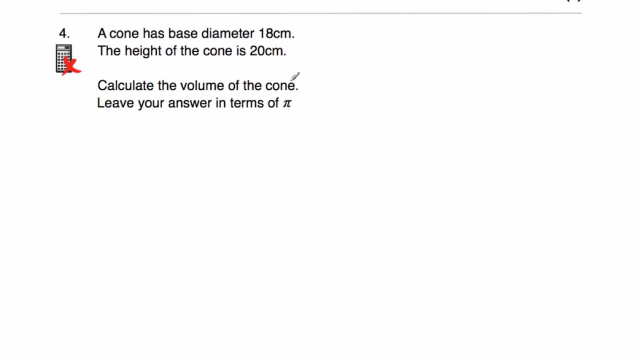 So we've got a base diameter of 18 centimetres and a height of 20 centimetres. Calculate the volume of the cone and leave your answer in terms of pi. So here I'm going to do a little sketch, So please excuse this. 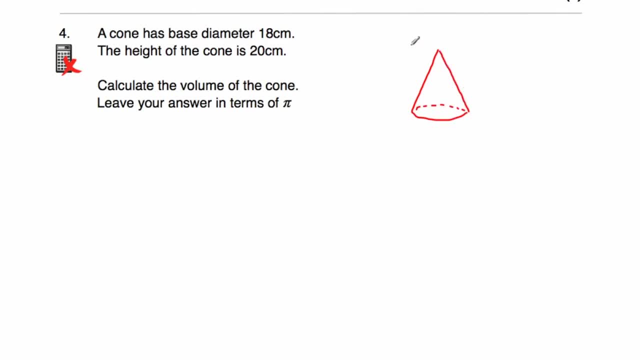 I'm doing it free hands. I might not necessarily be the best cone. So far, so good. There's my sketch of a cone and let's label it. We've got a diameter, So the diameter of the cone going from one side to the other side is equal to 18 centimetres and the height of the cone going straight up and down is equal to 20 centimetres. 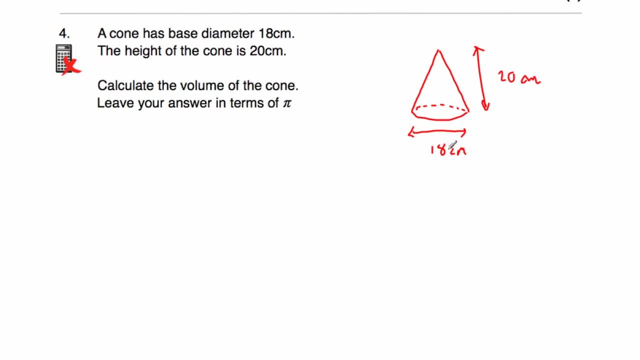 And we've been asked to work out the volume of this cone and to leave our answer in terms of pi. So it's a non calculator question. So let's write down The formula for finding the volume of a cone. So the volume is equal to a third pi r squared h. 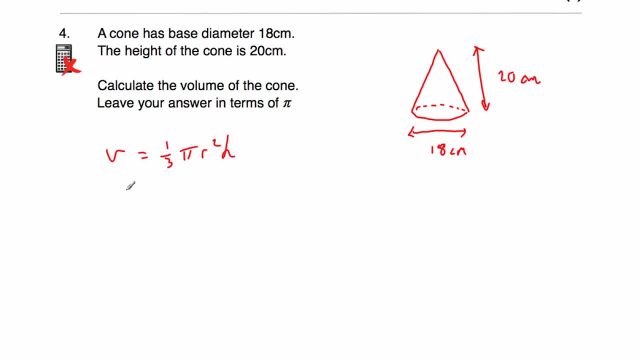 In other words a third times pi, times the radius squared, times the height. So let's substitute in our values that we know. So we've got a third multiplied by pi, multiplied by the radius squared. Now the diameter of the circle is equal to 18 centimetres. 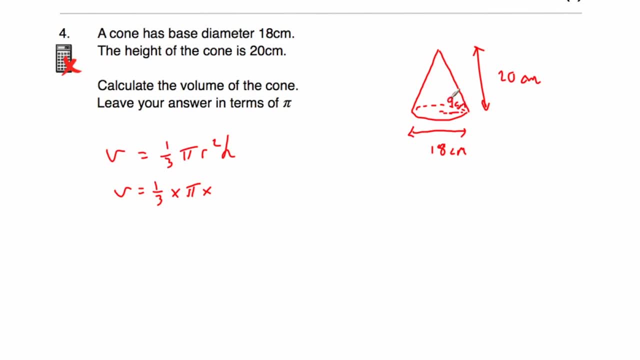 So the radius halfway across would be equal to nine centimetres. So the radius is equal to nine. So nine squared multiplied by the height and the height is equal to 20.. And now we need to work this out without a calculator. So we've got: the volume is equal to. 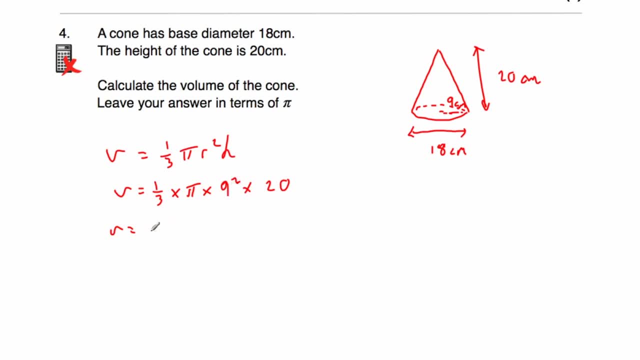 Now remember to do your squared first of all. So nine squared is equal to 81.. So we've got a third multiplied by pi, multiplied by 81, multiplied by 20.. So I'm going to do 81 times a third, to begin with. 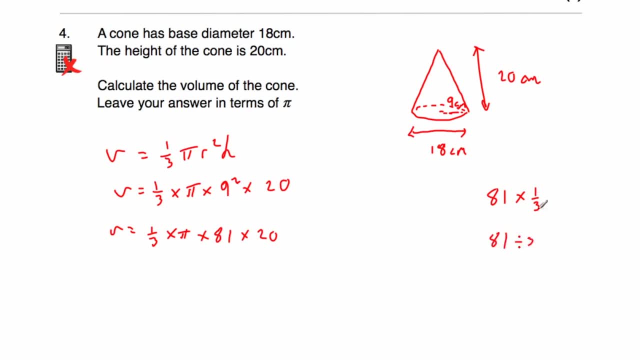 Or I'm just going to do 81 divided by three, because that's the same as multiplying by a third. So 81 divided by three. So 81 divided by three. Three into eight goes twice. Remainder two And three into 21 goes seven times. 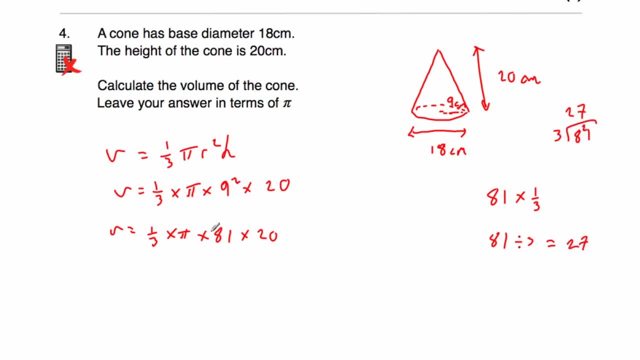 So 81 divided by three would be 27.. So that means that 81 times a third Is 27.. So we've got: volume is equal to 27 times pi times 20.. So we've just done a third times 81.. 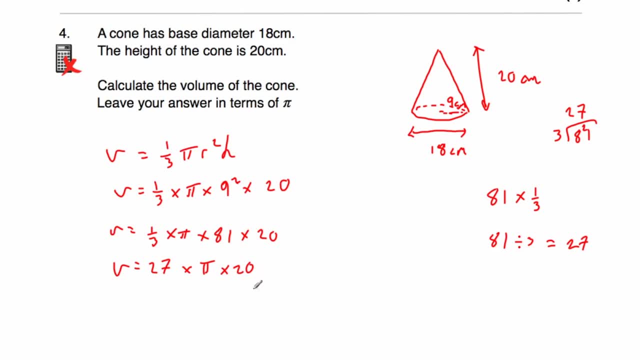 We've still got the times pi times 20.. So we now need to do 27 times 20.. So we could use the column method for that. We could do 27 times 20 and get our answer. Or another way to do it is: instead of multiplying by 20, we could times by two and then times by 10.. 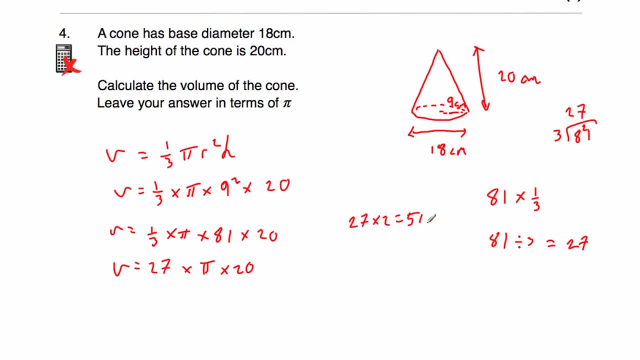 So let's take our 27 and multiply by two. That's going to be equal to 54. and then take our 54 and times by 10, and that's equal to 540.. So 27 times 20. Is equal to 540. 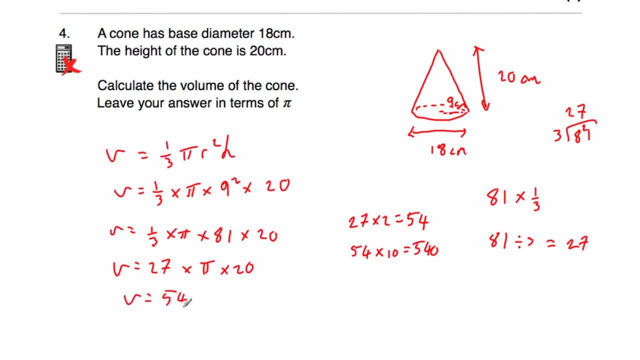 And we've still got the times pi. So volume is equal to 540 times pi. So the volume will be equal. to remember, we're just going to leave our answer in terms of pi, So we're just going to put them together. 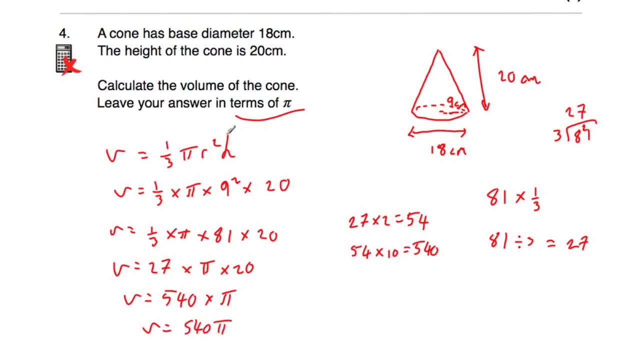 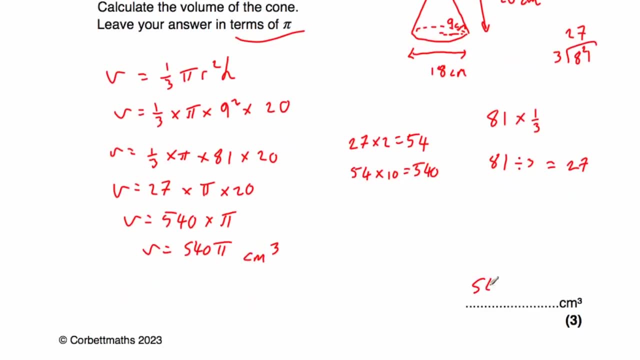 So it'll be 540 pi and we need to make sure we put on our units. That's the volume of the cone. We're dealing with centimeters, So it's going to be centimeters cubed. So the volume of this cone would be equal to 540 pi, centimeters cubed. 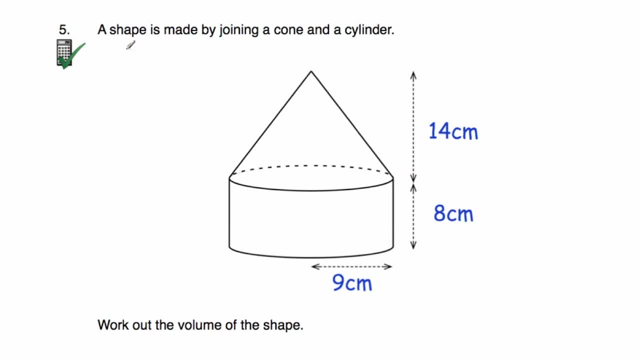 And that's it. Okay, Let's look at our next question. Okay, Let's have a look at question number five. We're going to be joining a cone and a cylinder. So here we've got a cone on top of a cylinder and we've been asked to work out the volume. 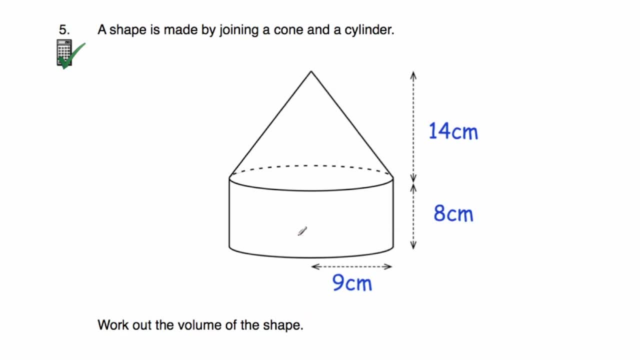 of the ship. So we need to work out the volume of the cone, We need to work out the volume of the cylinder and then add them together to get the volume of the whole ship. So let's start off with the code. So the code: the volume of a cone is equal to volume, is equal to a third pi R squared. 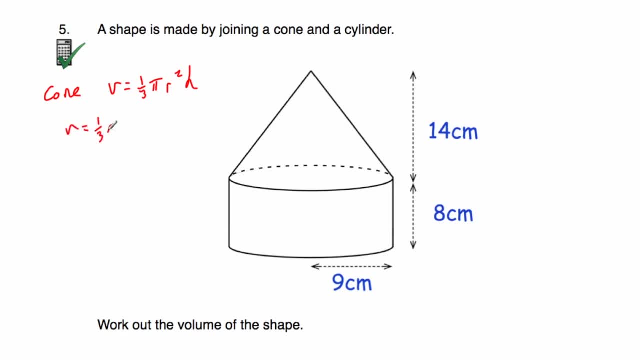 H. So we're going to do. the volume is equal to a third multiplied by pi, multiplied by the radius, And if we have a look at this code we know it's radius. So this distance from the center to the edge will also be equal to nine centimeters. the 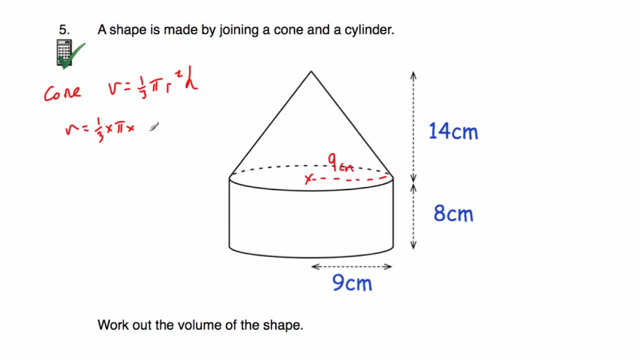 same as the radius- Okay, Okay, Okay, Okay, Okay, Okay, Okay- As the radius of the cylinder. So that's going to be multiplied by nine squared, multiplied by the height of the cone, and the height of the cone is equal to 14.. 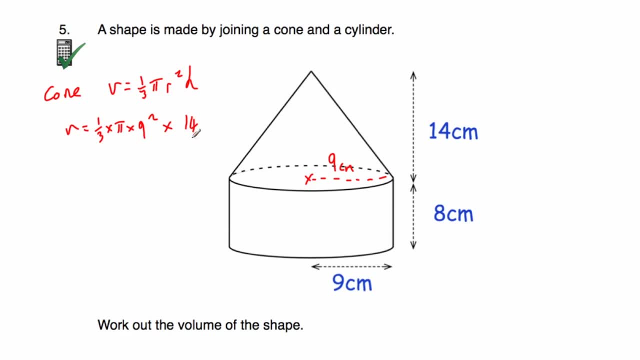 So if we do a third, multiplied by pi, multiplied by nine, squared, multiplied by 14, that would tell us the volume of this cone, and it's a calculator question, So let's type that in, And when we do that we get an answer of 378 pi centimeters cubed. 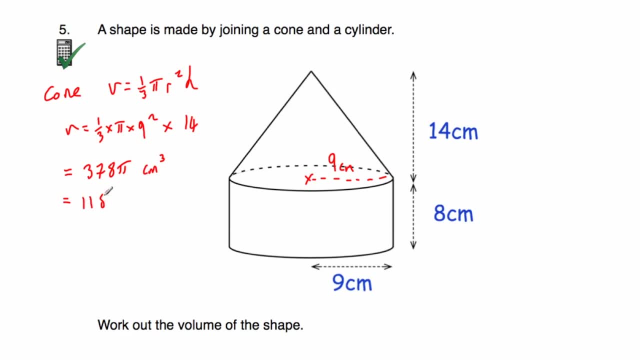 Alternatively, we could write it as a decimal number as 1,187.522023 and so on centimeters cubed. So we could write that, as the volume of this cone is either 378 pi or 1,187.522023, and so, 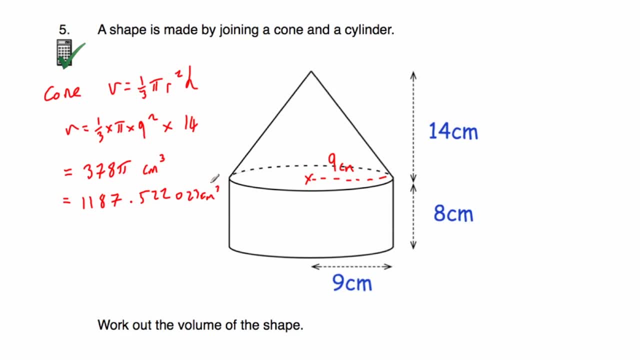 on centimeters cubed. So that's the volume of the cone. Let's find the volume of the cylinder. So the cylinder, So the volume of the cylinder, is pi R squared H. So we find the area of the circle, the area of the base, and then multiply by the height. 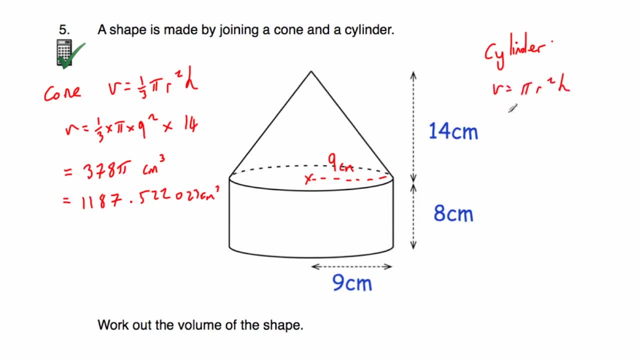 So the volume is equal to pi R squared H. So what we're going to do is we're going to do pi multiplied by the radius of the cylinder. So if we have a look at the cylinder, the radius, the distance from the center to the 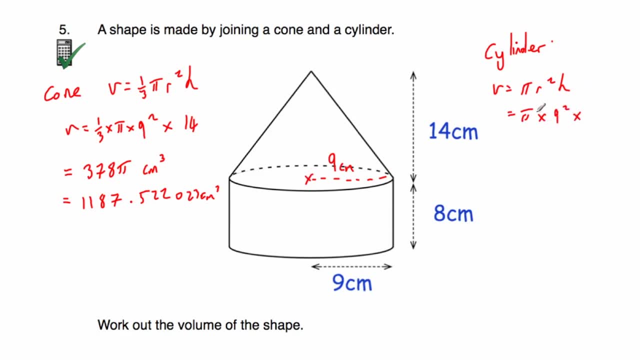 edge is 9. so we're going to multiply by 9, squared multiplied by the height of the cylinder. and the height of the cylinder is 8 centimeters, so multiply by 8. so we just need to do pi times 9, squared times 8, and when we do that we get that's equal to 648 pi centimeters cubed. so that's in terms of 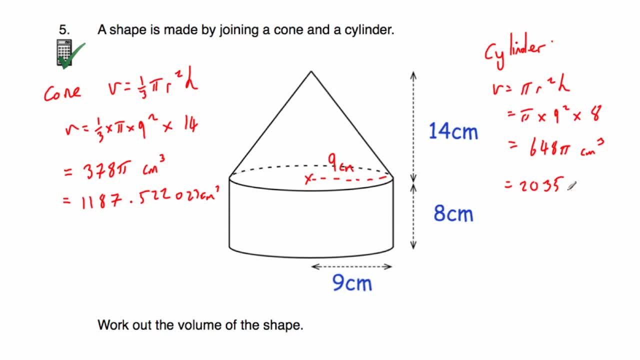 pi. alternatively, we could write as a decimal: that'd be 2035.75204 centimeters cubed. so we now know the volume of the cone, which is either 378 pi or 1187.522, and so on, centimeters cubed. and we've got the volume of the cylinder, which is either 648 pi or 2035.752, and so on, centimeters. 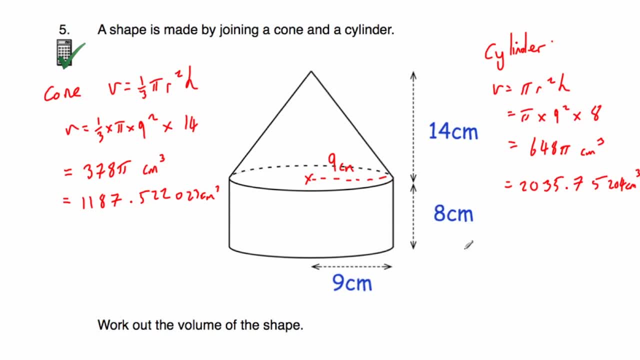 cubed. now we're going to then add them together to get the volume of the whole ship. so let's do that now. we can even do that in terms of pi. so we could do 378 pi plus 648 pi and then press equals and see what we get, and that's equal to 1026 pi. 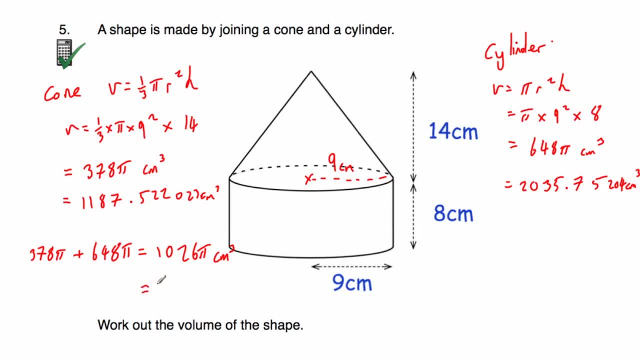 centimeters cubed. so that's the answer in terms of pi, and then you can convert that into decimal to be three thousand two hundred and twenty three point two, seven, four, zero, six, three and so on, centimeters cubed. so you can do it that way, adding the answers in terms of pi. alternatively, you could: 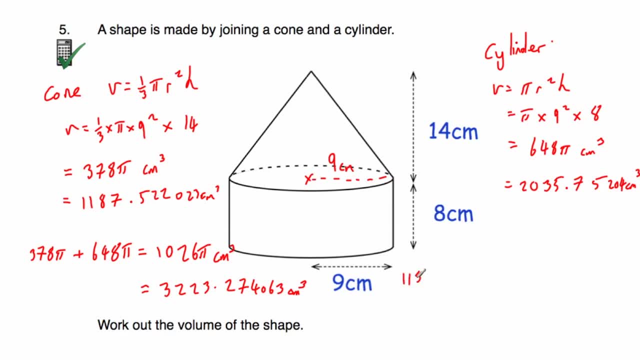 add these together so you could do your 1187.522023 and so on, centimeters cubed, plus our 2035.75204, and we can add those together and see what we get. when we do that, we get an answer off. now, depending on how you've typed it in, whether you use the memory on your calculator, you could have. 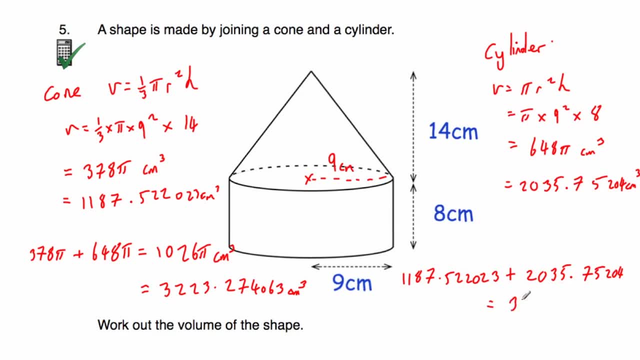 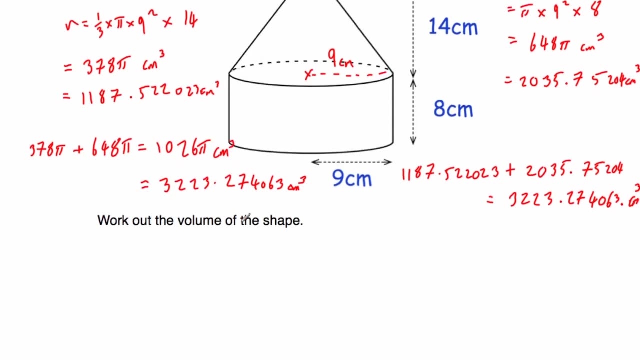 got 1026 pi or might just come up as 3223.274063 and so on, centimeters cubed and that's the same answer, and that's it. so the question says: work out the volume of the shape. so we could give our answer as 1026 pi, because it doesn't say to give it to so many decimal places, or i'm going to give. 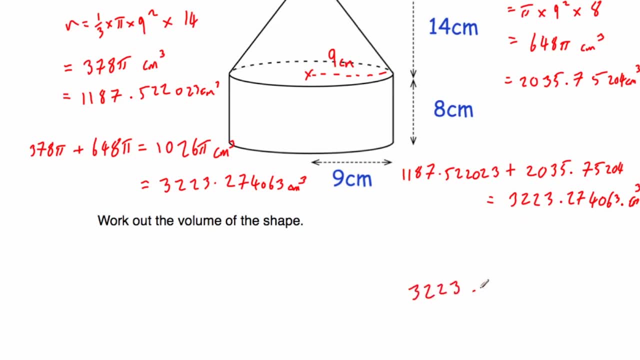 it as a decimal number. i'm going to give it as three thousand two hundred and twenty three, 274 centimeters cubed to three decimal places, and that's it. so that's the volume of that ship. okay, let's have a look at question number six. so, question number six: we've been given a cone. 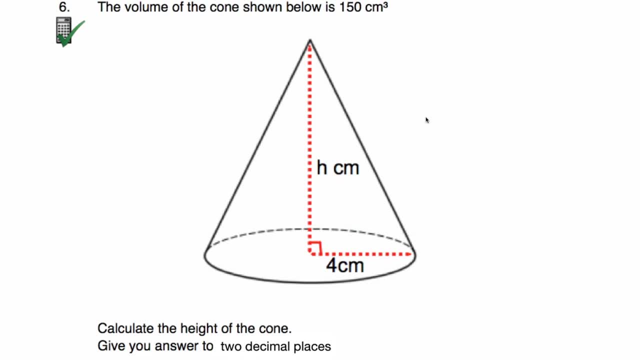 and we'll be told. the volume of the cone shown below is 150 centimeters cubed. so we've got the volume of this cone and we need to calculate the height of the cone and to give our answers to two decimal places. so it's a calculator question. so let's write down the formula: the volume of the. 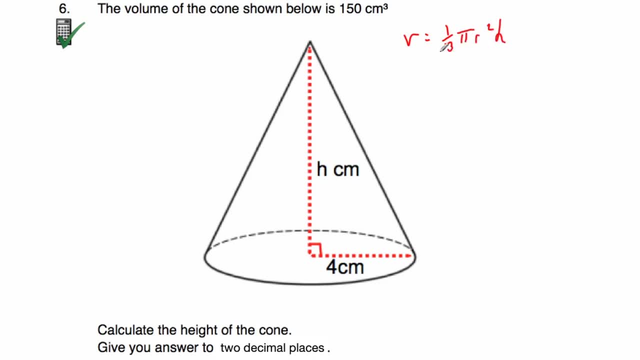 cone is equal to 3r squared h. now let's substitute what we know. we know the volume is equal to 150. so to write 150 equals instead of volume, or instead of the v, we're around 150. and then we've got a third: multiply by pi, multiply by the radius squared, but the radius is four. so multiply by. 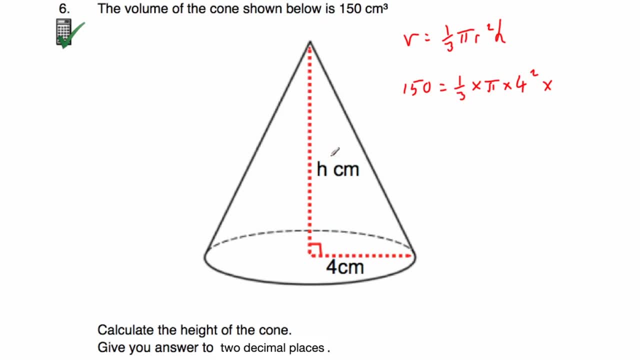 four squared, multiply by the height, and the height of this cone is equal to h. so we're going to put multiply by h. so now we've got an equation that we want to solve. we want to find the value for h, so we want h equal something. at this point we've got a few different approaches we could square. 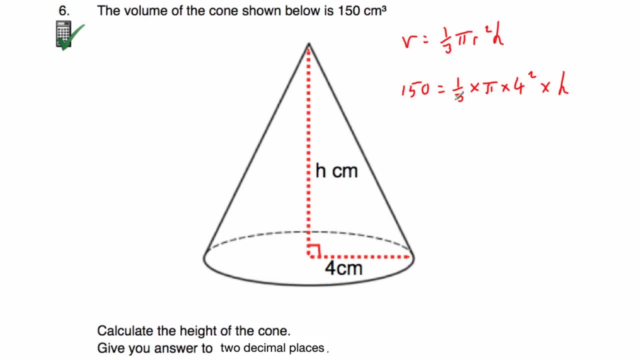 the four, and then we could divide both sides of the equation by a third, and then divide both sides of the equation by pi, and then divide both sides of the equation by 16, and that'll give you the value for h. now, because this is a calculator question, what i'm actually going to do is just 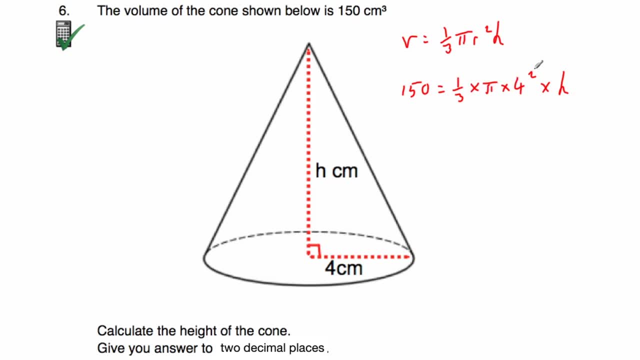 type into my calculator a third times pi, times four squared and that will just give me the number that we're multiplying h by. so when we do that we get- on the left hand side we've still got the 150. and on the right hand side, whenever we do a third multiplied by pi, multiplied by four squared, we get 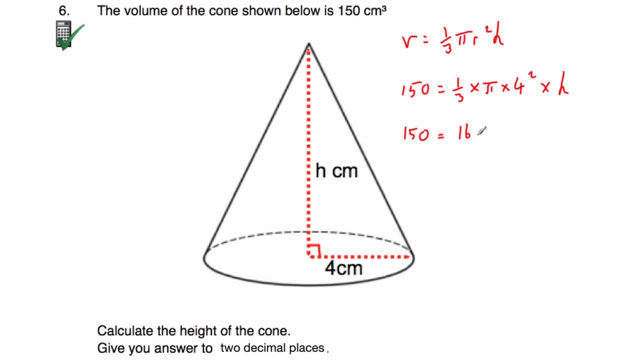 an answer of 16 over 3 pi, or 16.75516 and so on. and then we're going to divide both sides of the equation by pi and then divide both sides of the- we're still times in that- by h, so times by h. now we want to get the h on its own, so we don't want. 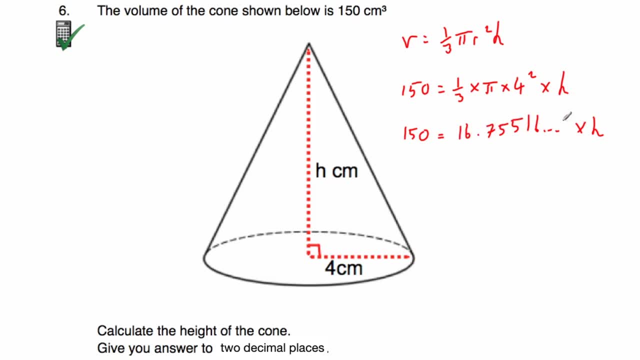 this multiplied by 16.75516, and so on. so what we're going to do is we're going to divide both sides of the equation by 16.755, and so on. so we'll divide the left hand side by that, and we'll also 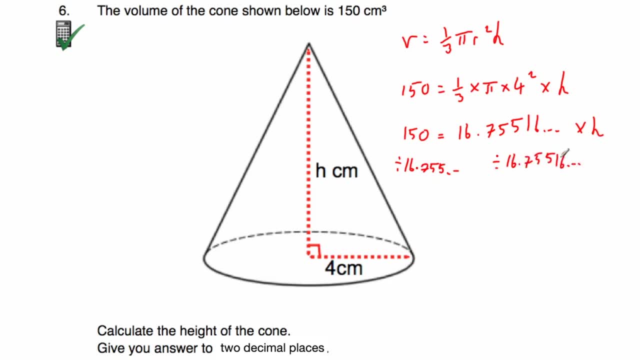 divide the right hand side by that, and that will leave us with just the h on its own. so whenever we divide 150 by 16.75 and so on, what i'm going to do is, on my calculator, i've still got my display, the 16.75516082. what i'm going to do is i'm going to press 150 and then just press, divide by and the. 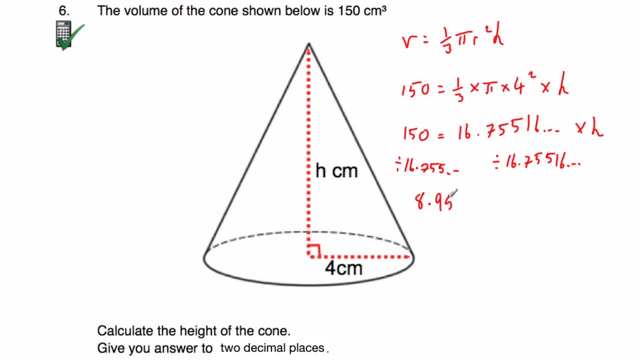 answer, and that will give me an answer of 8.95246 and so on. and that equals: and on the right hand side we had 16.755 and so on multiplied by h. we divided by the 16.755, and so on. so i'll just leave. 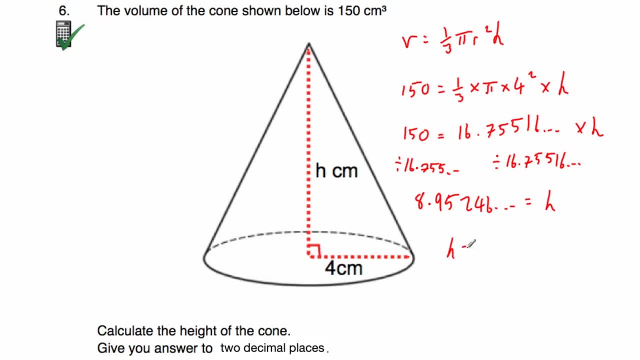 us with the h. so that's it. we've found the height of the cone. the height of the cone is equal to eight point nine, five, two, four, six and so on and so on, centimeters. now the question says to give our answer to two decimal places, so h, the. 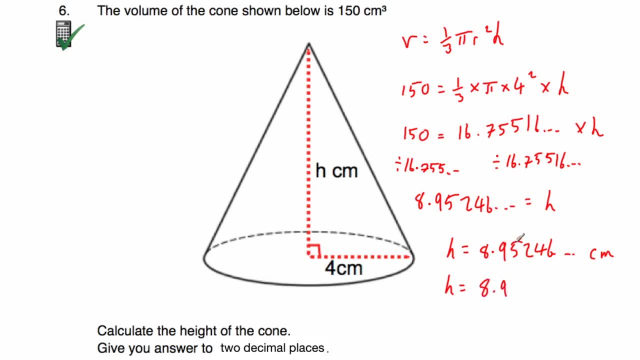 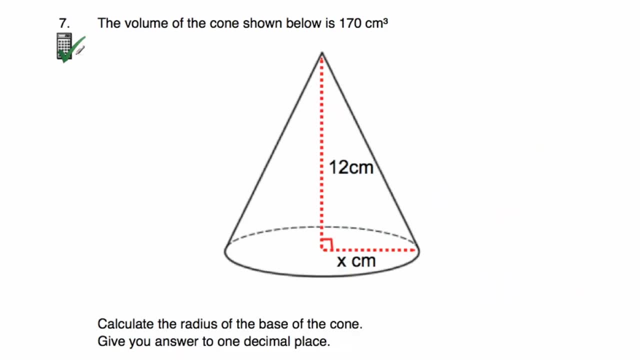 height of the cone is going to be eight point nine and if we have a look, we've got five two. so it's going to be eight point nine, five centimeters to two decimal places and that's it. okay, let's have a look at our next question. okay, let's have a look at question number seven. so question number: 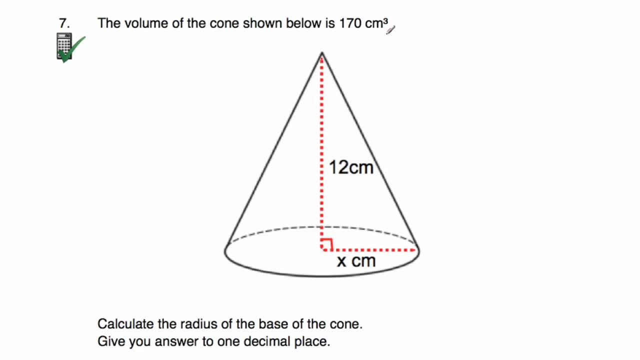 seven says the volume of the cone shown below is 170 centimeters cubed. so the volume of this cone is 170 centimeters cubed and we've been asked to calculate the radius of the base of the cone. so we want to calculate the radius of the cone. 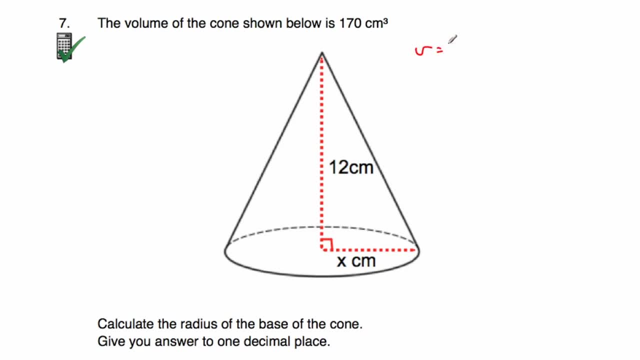 give our answer to one decimal place. so let's write down the formula. the volume is equal to a third pi r squared h. so the volume of the cone is a third times pi, times the radius squared multiplied by the height. so we know the height is equal to 12 and we know the volume is equal to 170. 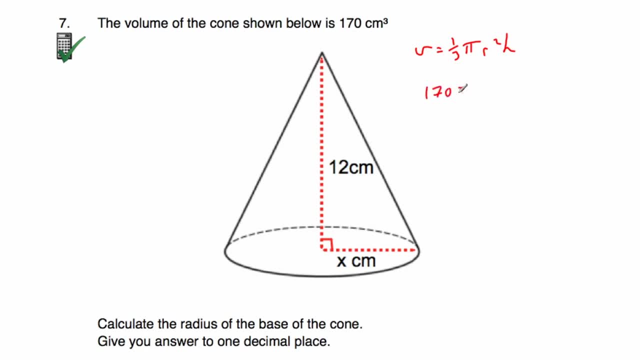 so let's substitute those in. so we've got 170 equals a third multiplied by pi, multiplied by the radius. now in this case the radius is x. i'm going to write x squared multiplied by the height, and the height is equal to 12. so now we've got an equation that we want to solve to find x. we want x. 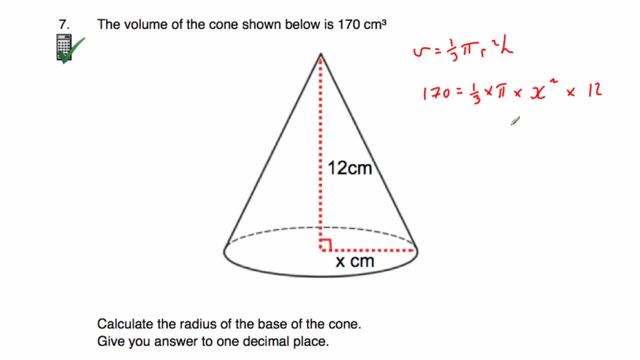 equals something. so at this point, what we could do is we could divide both sides of this equation by a third, we could divide both sides of the equation by pi, and we could also divide both sides of the equation by 12, and that will leave us something equals x squared, and then we could square root. 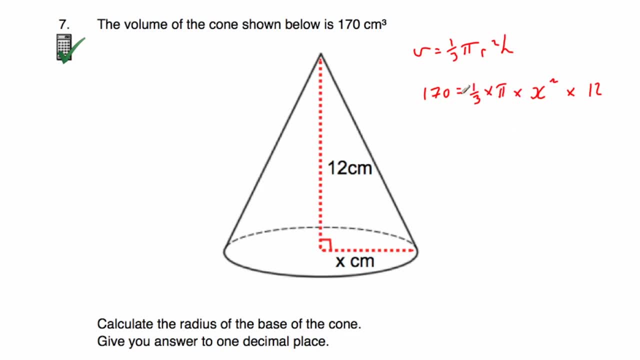 to find what x is. so that's one approach we could use in this case. what i'm actually going to do is i'm going to leave the left hand side as it is. i'm just going to write 170 and on the right hand side, what i'm going to do is i'm going to multiply the third, the pi and 12 together, to see. 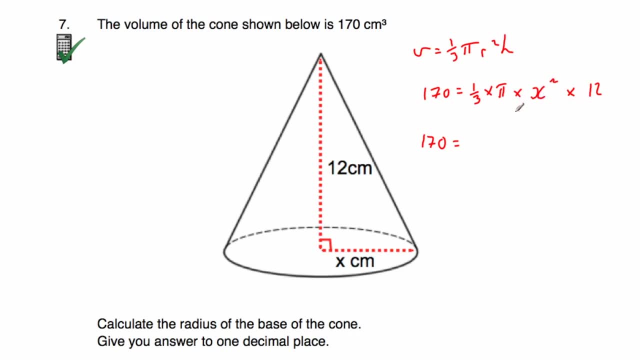 what number we're multiplying x squared by. so if we on our calculator type in a third multiplied by pi, multiplied by 12, and that's equal to 4 pi, or as a decimal number 12.5663 and so on, and we're still multiplying that by x squared, so we've now got 170 equals 12.5663 and so on multiplied by x. 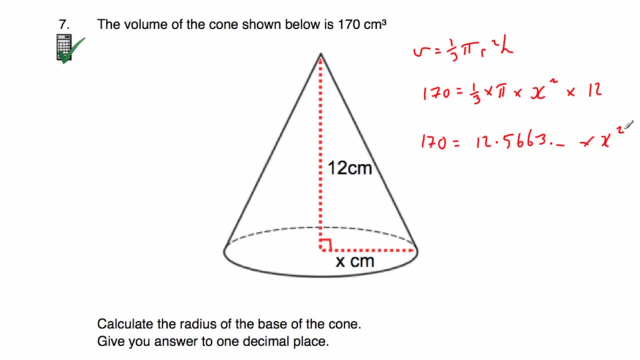 squared, or 170 equals 4 pi multiplied by x squared. so now we want to get the x on its own, so we want to get rid of this multiplied by 12.5663 and so on. so let's divide the left hand side of the equation by 12.5663 and so on, and let's divide the right. 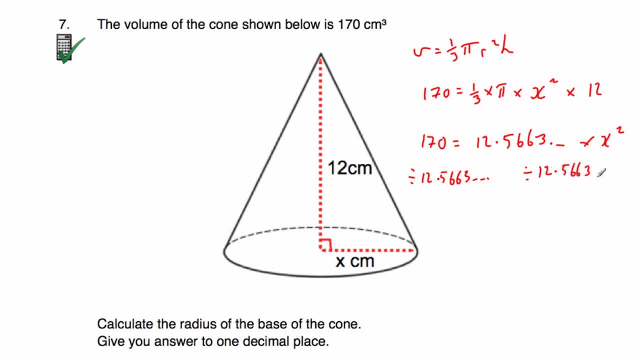 hand side of the equation by 12.5663 and so on. or you could have just divided by 4 pi and 4 pi, and when we do 170 divided by 4 pi or the 12.566 and so on, we'll type in 170 divided by answer, and 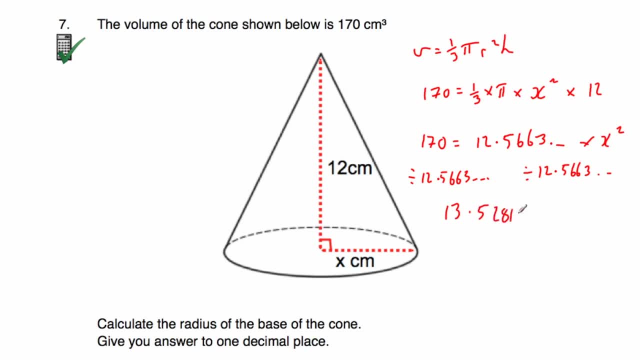 we get that's equal to 13.52817 and so on, and that's equal to: and on the right hand side we had multiplied by x, squared, we divided by the 12.5663, and so on, to get rid of it. so we'd just be left. 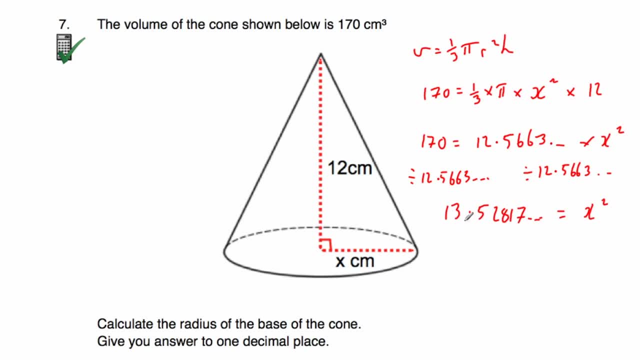 with x squared. so we've now got the x squared is equal to 13.52817, and so on. now we don't want x squared, we just want to find x. so we want to get rid of this squared now, because x is going to be. 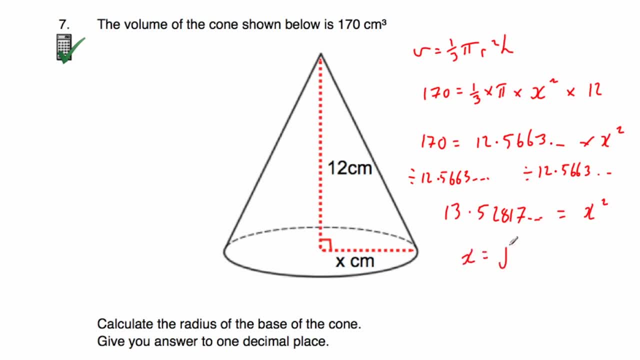 positive number. we can just square root this. so we're going to find x is equal to the square root of 13.52817 and so on, and when we work out the square root of that, we get the x is equal to 3.6780.. 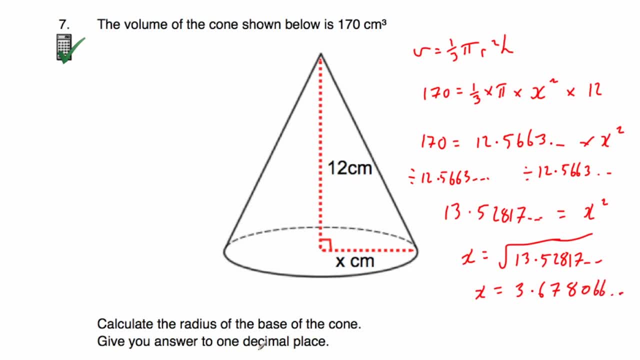 zero, six, six and so on. now the question says to give our answer to one decimal place. so that means the one decimal place that X will be equal to three point seven centimeters, and that's it. so the radius of this cone is three point seven centimeters to one decimal place, and that's it. so question break we've. 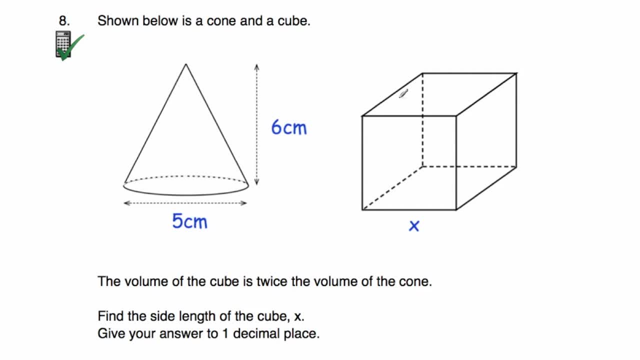 got our cone and a cube and we're told the volume of the cube is twice the volume of the cone. so the volume of this cube is twice double the volume of this cone. and we've been asked to find the side length of the cube, X. so what we 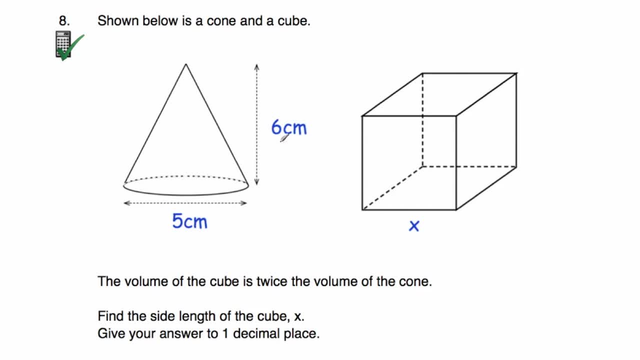 want to do here is we want to find the volume of the cone to begin with. we're gonna then double it, now be the volume of the cube, and then we want to find the side length, so we'll cube root because remember the side times, the side times. 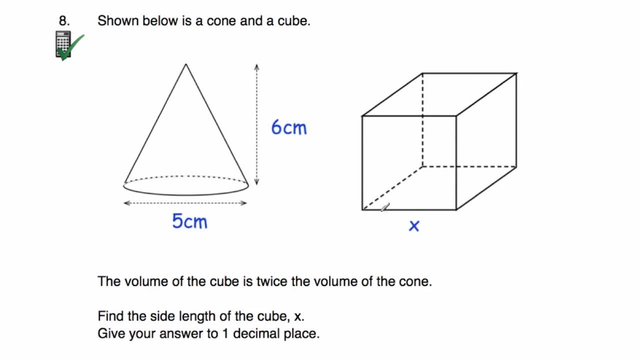 the side. the length times the width times the height is equal to the volume because there's a cube. they're all the same. so we know the X cubed will be equal to whatever double your volume of this is. so if we cube root it that'll. 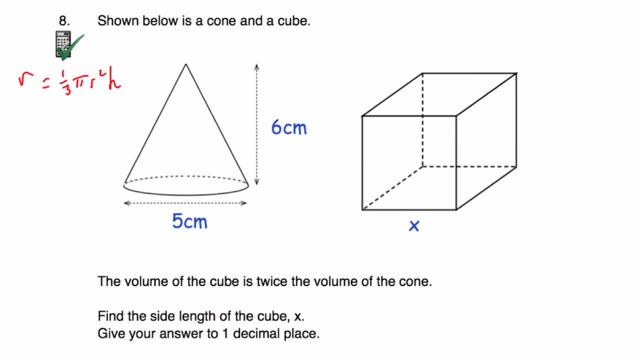 just give us this length here, X. so let's find the volume of the cone to begin with. so the volume of the cone is equal to a third pi R squared H. now if we have a look at our cone, we know the height. the height is equal to six and in terms 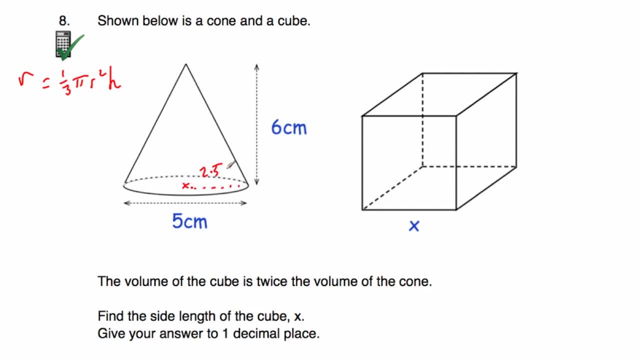 of the radius. the radius would be equal to two point five, so the radius of the cone would be equal to two point five centimeters. so we're gonna substitute in two point five for the radius and six for the height, and then that would give us whenever we 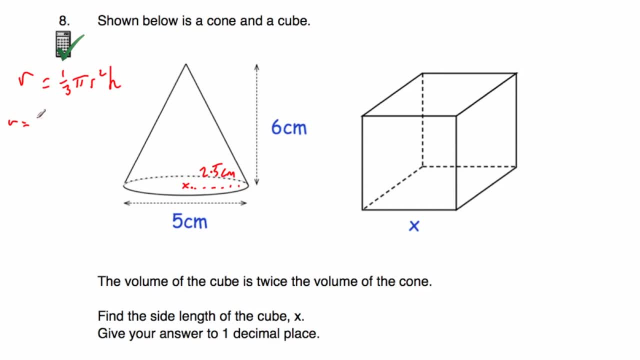 work it out, the volume of the cone- so it's going to be equal to volume- is equal to a third multiplied by pi, multiplied by two point five squared, multiplied by the height of the cone, which is equal to six. and whenever we do that on a calculator we get that's equal to 25 over 2 pi centimeters cubed, or as a 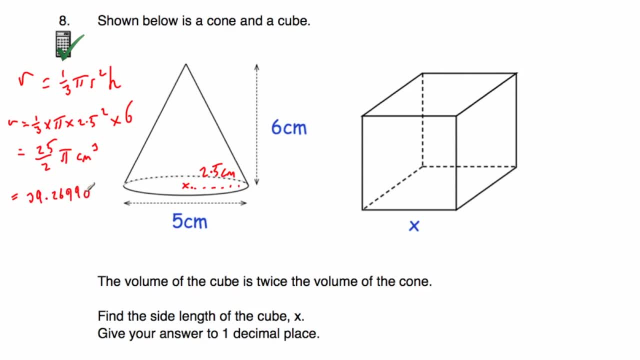 small number. we could write thirty nine point two, six, nine, nine zero eight one seven centimeters cubed. so that's the volume off the cone and the volume of the cube is twice the volume of the cone. so we now need to multiply the volume off the cone by two to get the volume off the cube. so that means for the cube its 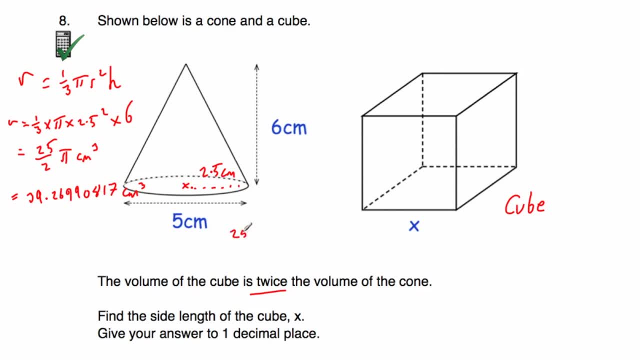 volume will be this multiplied by two. so we're gonna do our either 25 over 2 pi times by two and get our answer, which would be 25 pi centimeters cubed, or we could do our thirty nine point two, six, nine, nine, zero, eight, one, seven and multiply that by two, and then that would 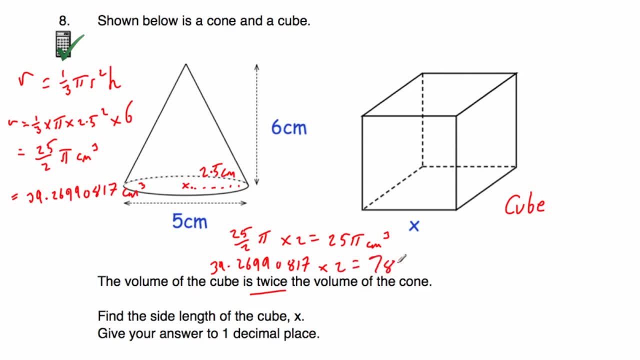 hopefully come up with 25 pi as well, or you could change it to a decimal, which would be seventy eight point five, three, nine, eight, one, six, three, four. and it's very important that if you're working in decimal so you don't run these answers until the very, very end, because if you run them too early it can introduce an. 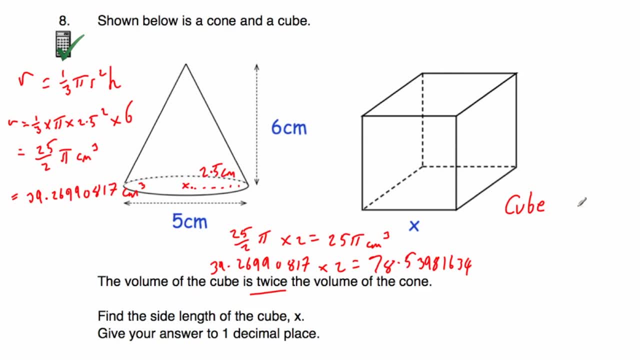 error into your your answer. so here we've got: the volume of the cube is equal to 25 pi, or this number. so that's the volume. now remember, here we've got X times the height, so X cubed is equal to 25 pi. or we could write down our seventy. 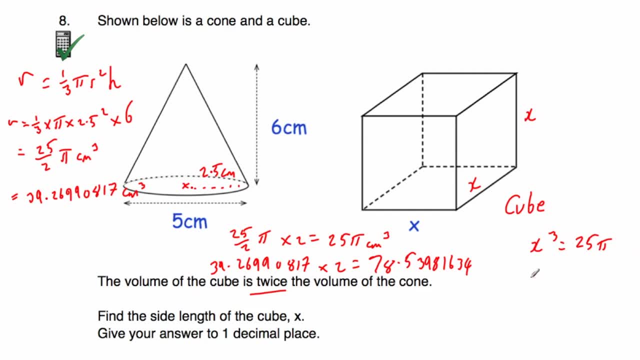 eight point, five, three, nine and so on, and then we just need to cube root. so if we do the cube root of 25 pi or your seventy eight point, so what, that would tell you X. whenever we do the cube root of that- and I've got that on my 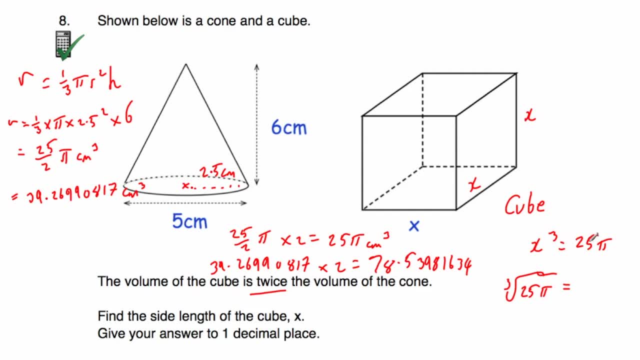 calculator display so I can just press the cube root of answer and that's equal to, and I get four. point two, eight, two, four and so on centimeters. so that is the length of X, point two, eight, two, so on centimeters. and this question we're asked to give. 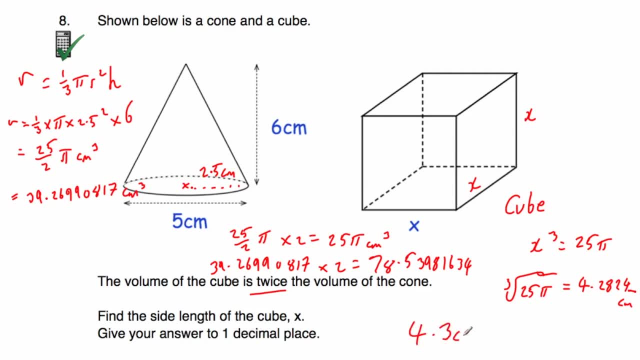 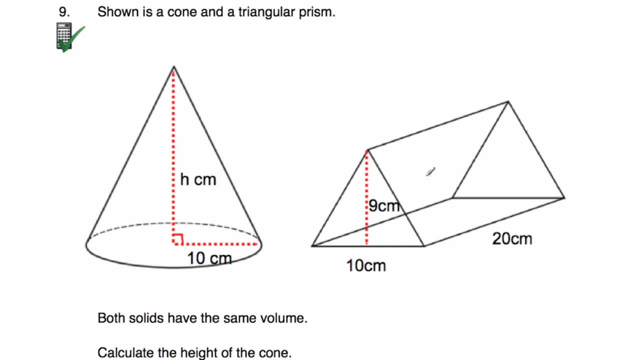 an answer to one decimal place. so answer be four point three centimeters, and that's it okay. let's look at our next question, question number nine. so question number nine says: shown as a cone and a triangular prism. so we've got a cone and a triangular prism and let's scroll down a little bit and we're told: 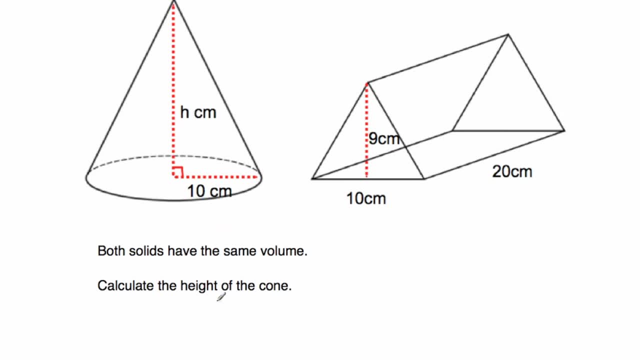 both solids have the same volume, so the volume of them is the same. I've been asked to calculate the height of the cone, so let's start with the triangular prism. let's find the volume of this triangular prism, because I've got the same volume. if we can work out the volume of this, that would be equal to: 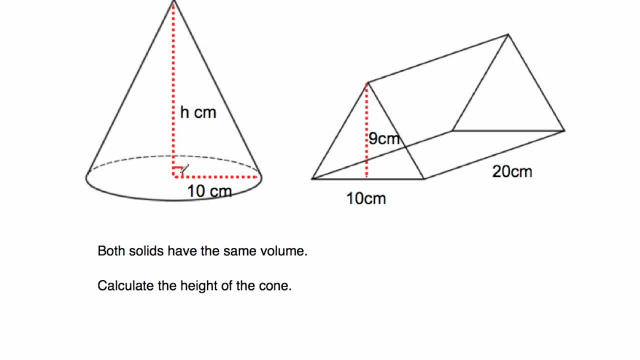 the volume of that and then, if we know the volume of this, we can then work out its height. so let's start off with the triangular prism. to get the volume of triangular prism, what we need to do is find the area for the triangle and then just multiply by how long the shape is. so if we find the area for the triangle, 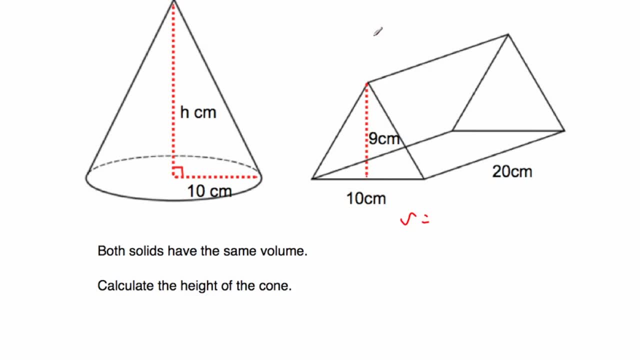 so the volume would be equal to half the base times. the height would be equal to half of 10 multiplied by 9. half of 10 is 5 times 9 is equal to 45 centimeters squared. so there, if that triangle would be 45 centimeters squared, you could do. 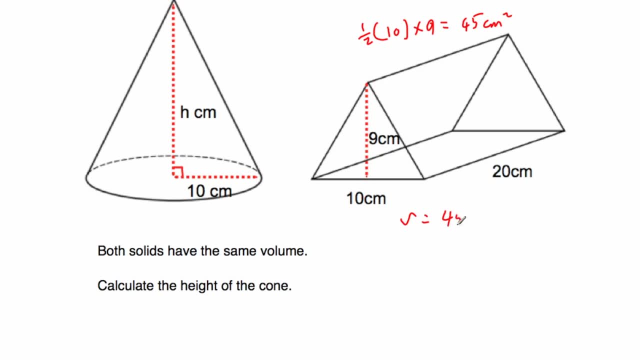 10 times 9 is 90, and then half it's 45. so we've got 45 for the area for the front, and then we just need to multiply how long the shape is. so multiply by 20 because there's a prism. so 45 times 20. 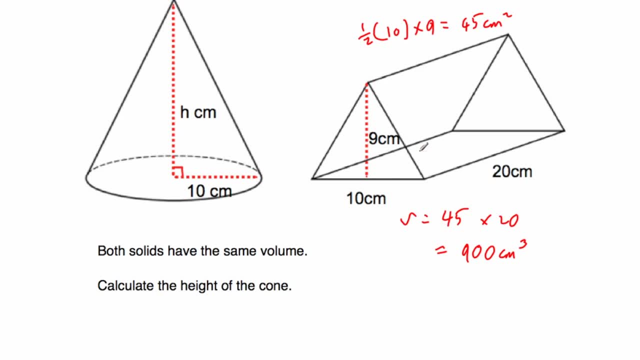 would be equal to 900 centimeters cubed. so that's the volume of the triangular prism. so that's the volume of the cone. so the cone has a volume of 900 centimeters cubed and we want to find its height. so let's go scroll down a. 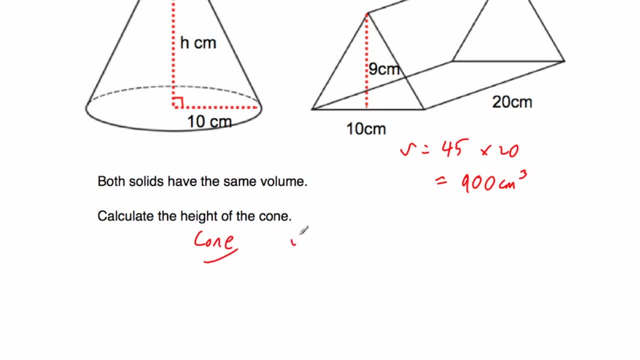 little bit. so for the cone the volume of the cone volume is equal to third pi R squared H, and we know that the volume is equal to 900. so let's substitute that in 900 is equal to a third times by pi, times by the radius, which is 10 squared. so multiply by 10 squared, multiplied by the height. 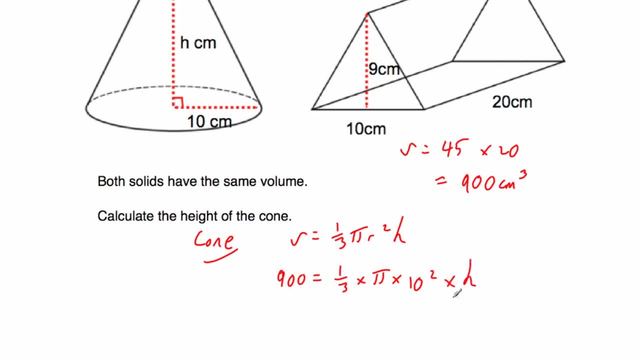 which is H, and we just need to solve this. this is an equation. we just want to solve H and get H on its own. so at this point what we could do is we could work out what 10 squared is- that's a hundred- and we could divide both sides of this. 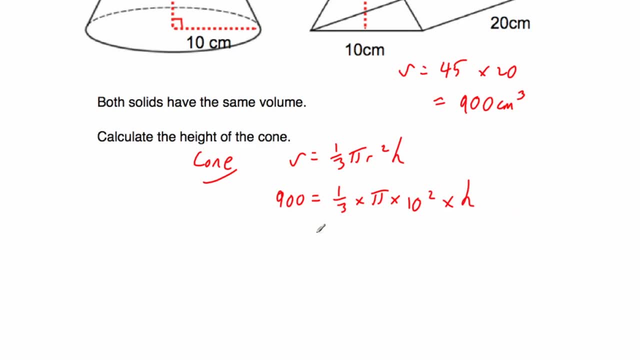 equation by a third and then divide both sides of the equation by pi, and then divide both sides of the equation by 100. and that would work now, because it's a calculated equation. what I'm actually going to do is I'm going to type a third. 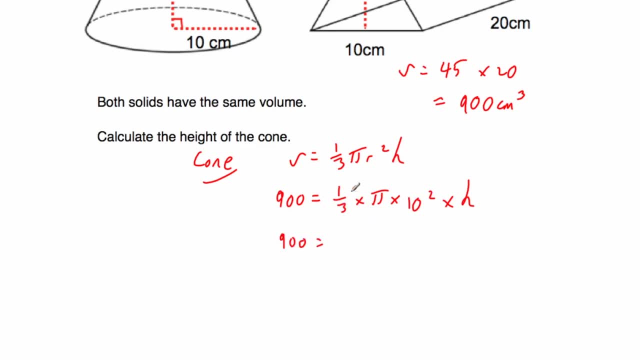 times 10 squared into my calculator, and I'm gonna see what that's equal to. whenever I type that in, I get that's equal to 100 over 3 pi, or 104.7197 and so on, and then we've still got R multiplied by H. so whenever we work out a third, 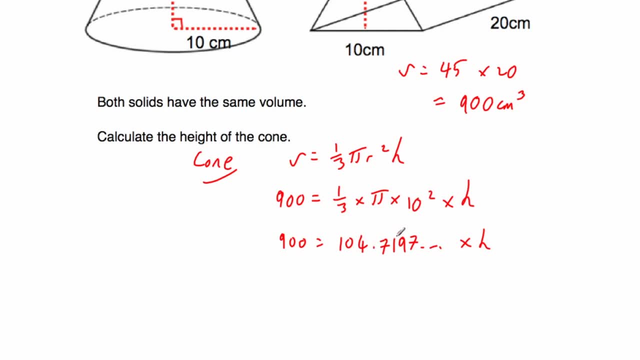 times pi times 10, squared, that's equal to 104.7197 and so on. and we want to find what H is. so we don't want this multiplied by 104.7 and so on. so what we're going to do is divide both sides of the equation by that. so we're going to. 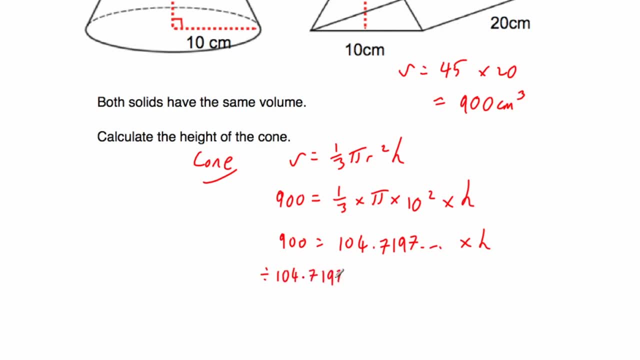 divide both sides by 104.7197 and so on and divide the left hand side by it and the right hand side, and whenever we divide both sides of the equation by that, on our left hand side we'll just do 900 divided by answer on our calculator and that will give us 8.5943669. 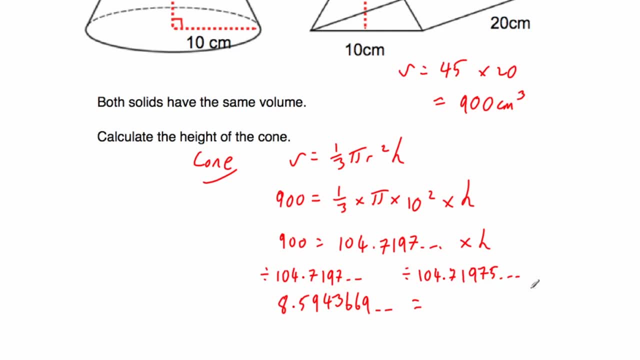 and so on. and on the right hand side we divided by 104.7 and so on to get rid of the multiply by 104.7, so on, so we're just left with our H. so we get the height of the cone. H is equal to 8.5943, and so on, centimeters, and 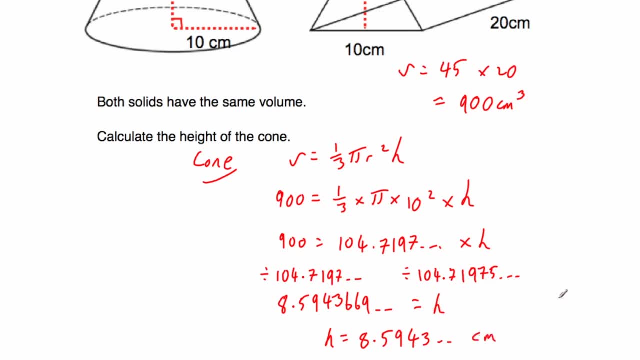 we could round our answer. let's round it to one decimal place. so the height of the cone to one decimal place would be 8.6 centimeters, and that's it. yeah, let's have a look at question number 10. so question number 10 says Jasmine has a. 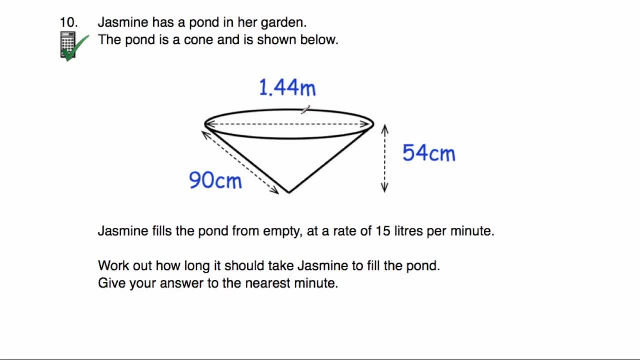 pond in her garden and the pond is a cone and is shown below. so this is the pond, so this is the surface of the pond and it goes down onto the ground like so, and it's got a diameter of 1.44 meters, it's got a height of 54 centimeters and 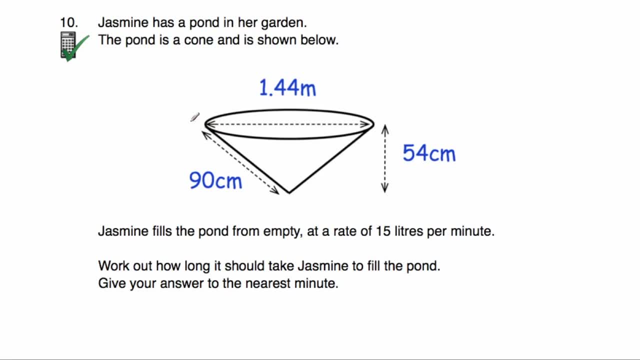 the slant height. so the length of the slants here is equal to 90 centimeters. and Jasmine fills the pond from empty. so it's empty and she fills it at a rate of 15 liters per minute. now remember one liter. one liter is equal to 1,000. 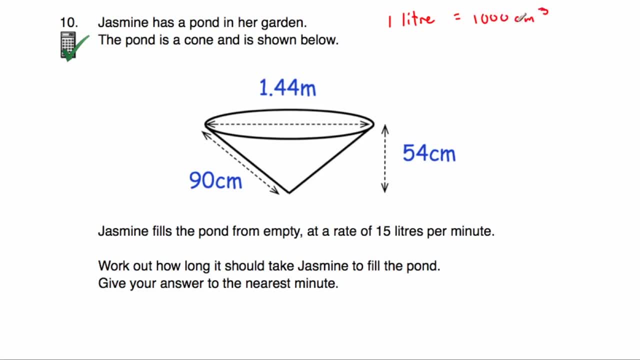 centimeters cubed. so that means that she's filling at a rate of 15,000 centimeters cubed per minute. and the question says: work out how long it should take Jasmine to fill the pond. give your answer to the nearest minute, so we want. 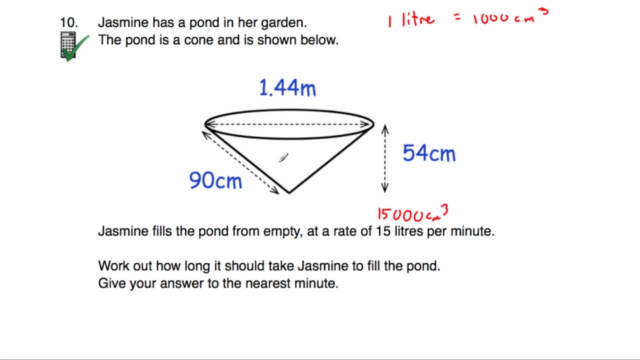 to work out, first of all, the volume of this cone. if we can work out the volume of the cone, we can then calculate the volume of the cone and then we can then see how long it should take her to fill it, because she's filling it at 15,000. 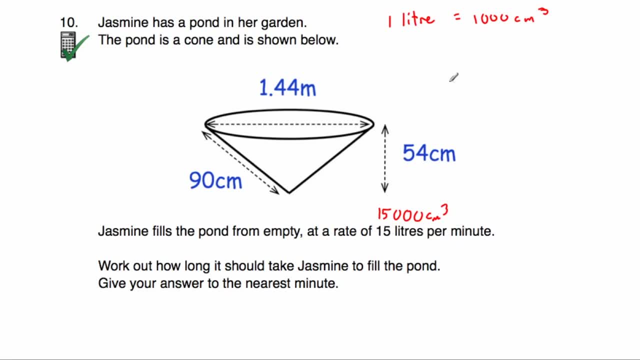 centimeters cubed per minute. so let's find the volume of this cone. so the volume is equal to 1, 3rd pi r squared h, and that's equal to 1, 3rd multiplied by pi, multiplied by the radius. now, because we know that we're filling at a rate of 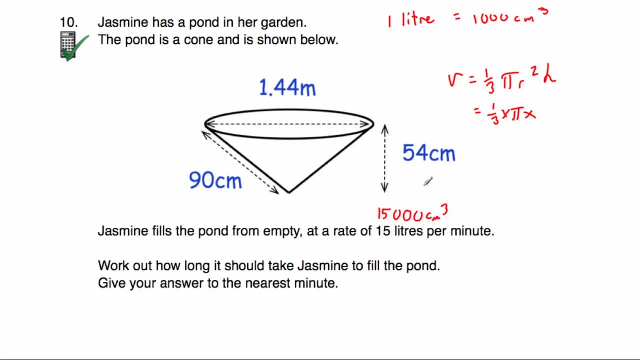 15,000 centimeters cubed per minute. I'm gonna work in centimeters in this question. so if the diameter is equal to 144 centimeters, if we half it, that'll be the radius of the cone. so 144 centimeters cubed per minute. so that's. 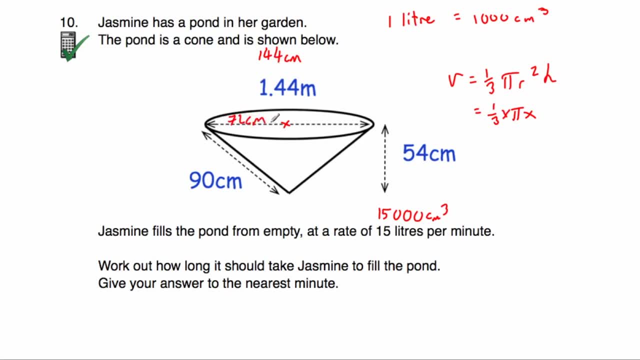 44 divided by 2 would be equal to 72 centimeters. that means the radius is equal to 72 centimeters. so we're gonna do a third times: pi times 72, squared times by the height, and the height is equal to 54. the perpendicular height: how? 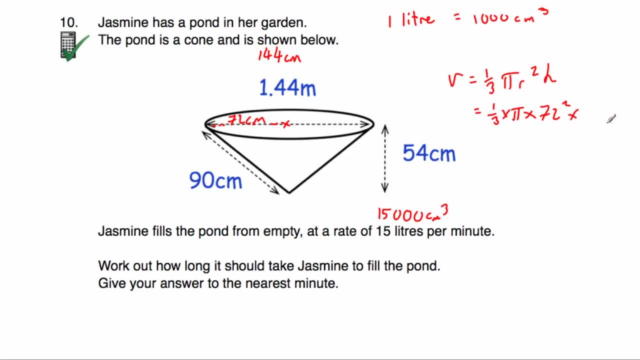 tall the cone is, or, in this case, I suppose, how deep the cone is, which is times by 54, and we're not going to be using the 19 this question. so what we're then going to do is: this is calculated a question, so we can type in one third. 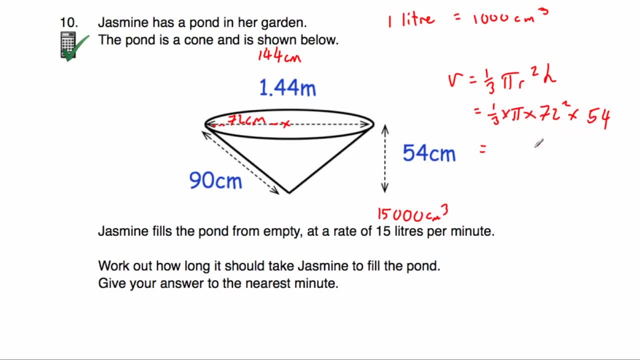 multiplied by pi, multiplied by 72, squared multiple up by fifty four, and if do that, we get an answer of 93,312 pi centimeters cubed. In this case, I'm going to convert that into a decimal number which is equal to 293,148.2937 centimeters cubed. So we've now got the volume. 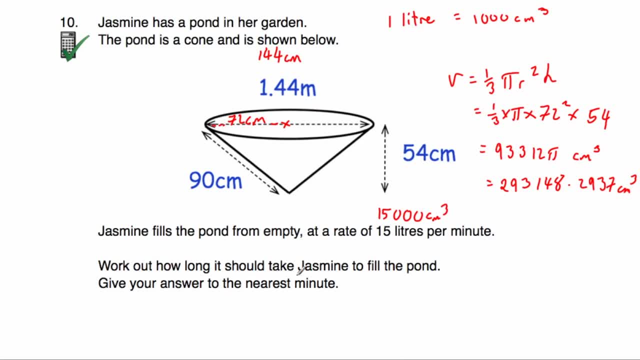 of the cone. Now the question asks us to work out how long it should take Jasmine to fill the pond. Give your answer to the nearest minute. So if we divide the volume by how many centimeters cubed are going in every single minute, we can then see how many minutes it should take. So if we do our 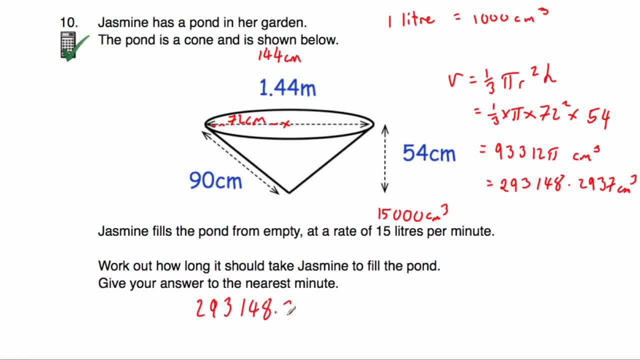 293,148.2937. and if we divide that by 15,000- because in every single minute 15,000 centimeters cubed of water is going into the pond- it tells how many minutes it should take. So whenever we divide by 15,000 we get an answer of 19.543, and so on minutes. Now the question says: give your 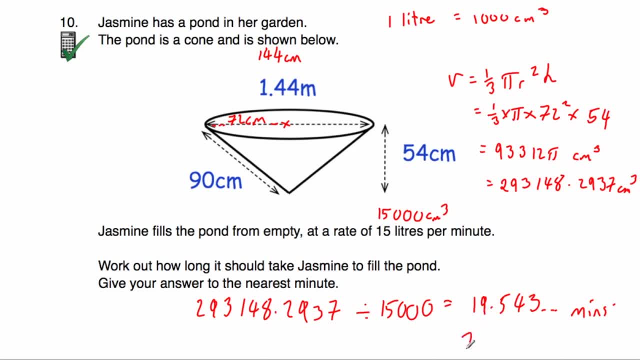 answer to the nearest minute, because it's 19.5. we're going to round up, So the answer would be 20 minutes. So, to the nearest minute, it will take Jasmine 20 minutes to fill the that pond with water, and that's it. Okay, let's have a look at our next question. So, 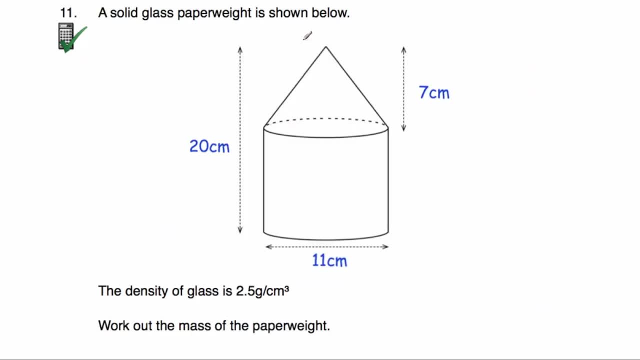 let's have a look at question number 11.. So question number 11 says the solid glass paper weight is shown below. So this is a glass paper weight. It's got a cylinder on the bottom bit of it and then we've got a cone on the top and we're told the density of the glass is 2.5 grams per. 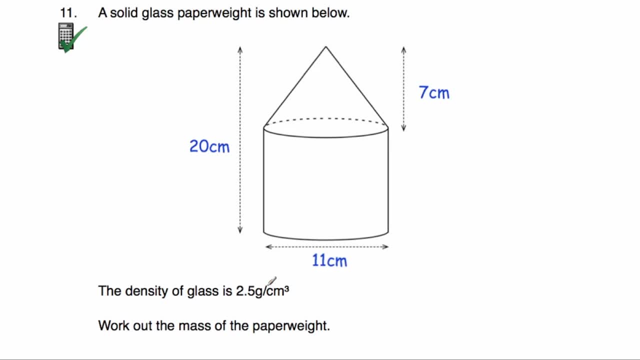 centimeter cubed. In other words, each centimeter cube has a mass of 2.5 grams. So we can find its volume. We can then just multiply by 2.5 and that will tell us the mass. Okay, so we need to find the volume of this paper weight. So we've got the cone and we've got the 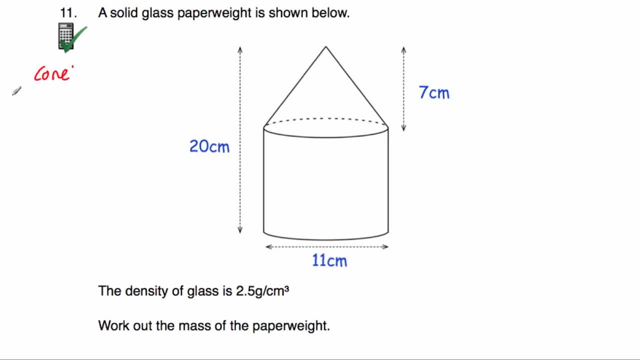 cylinder. So let's start off with the cone. So the cone we've got, the volume is equal to a third pi r squared h. So that's going to be: the volume is equal to a third multiplied by pi, multiplied by the radius. Now, the radius of the cone will be the distance from the edge to the center, which 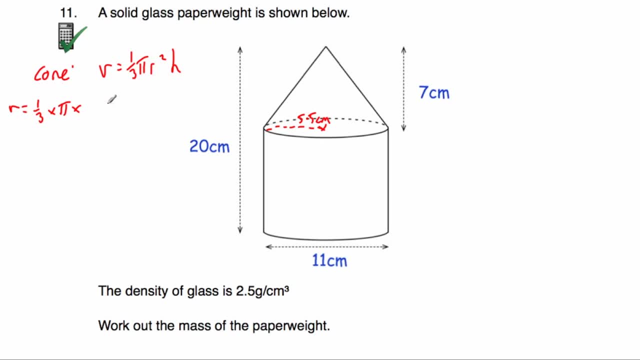 would be 5.5 centimeters, half of the 11. So multiply by 5.5, squared, multiplied by the height of the cone, which will be 7 centimeters, And when we do on our calculator, a third times, pi times 5.5. 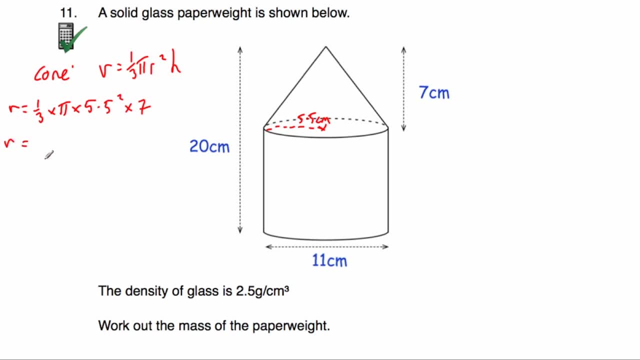 squared times 7, we get an answer of 847 over 12 pi, or 221.7440815 centimeters cubed. So that's the volume of the cone. Now let's deal with the cylinder. So the cylinder, the volume of the. 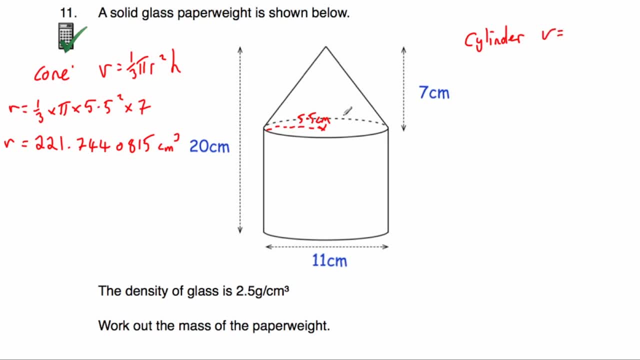 cylinder will be equal to the pi r squared there, the circle times by how tall the cylinder is. So the volume will be equal to pi times the radius of the cylinder, which again is 5.5. so 5.5 squared multiplied by the height of the cylinder. Now the height of the whole shape is 20 centimeters. The 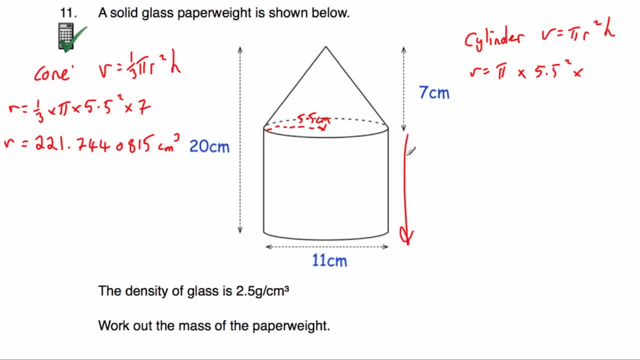 height of the cone is 7.. So if we do 20, take away 7, we'll get. the height of the cylinder is equal to 13 centimeters, So multiply by 13.. So if we do pi times 5.5, squared times 13, that will give us the 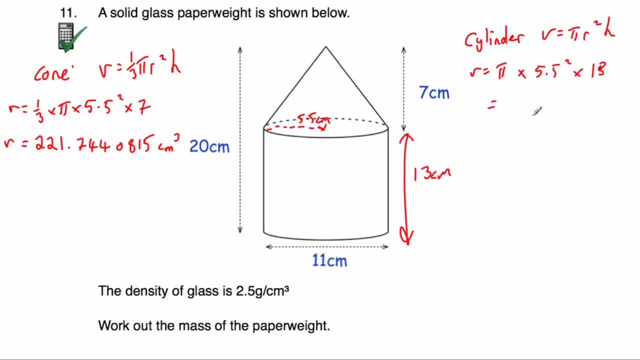 volume of the cylinder. So that's equal to 1573 over 4 pi over 12 centimeters. So that's equal to 4 pi over 12 centimeters, or 15235.431311 centimeters cubed. So that's the volume of the cone and. 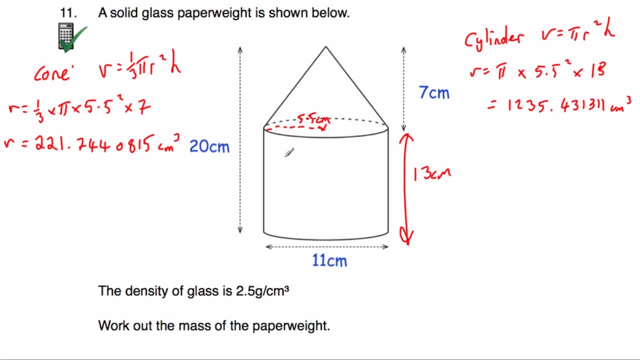 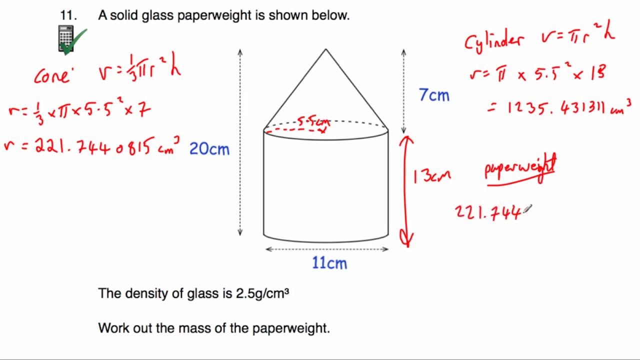 that's the volume of the cylinder And if we add them together that will be the volume of the paperweight. So for the paperweight to get its volume, we'll add these two volumes together, So we'll do 221.7440815 plus 1235.431311.. And when we do that we get. we get an answer of: 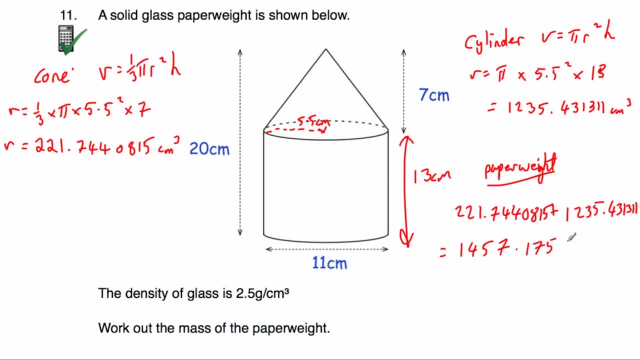 2457.175393 centimeters cubed. So that's the volume of the paperweight. Now we want to find the mass of the paperweight and we're given the density of the glass. Now we've got a couple of ways we can. 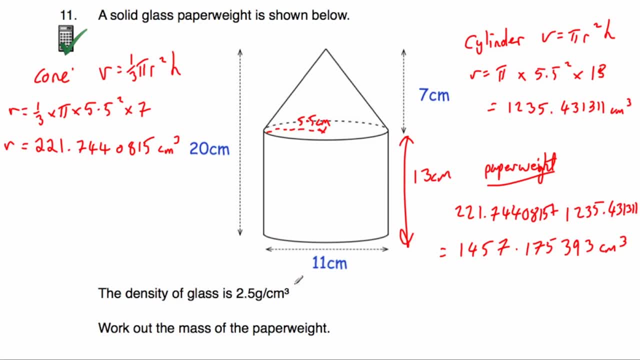 consider this. First of all, the density is saying that each centimeter cubed has got a mass of 2.5 grams. So if we just times the volume by 2.5, that will tell us the mass of the paperweight. So that's. 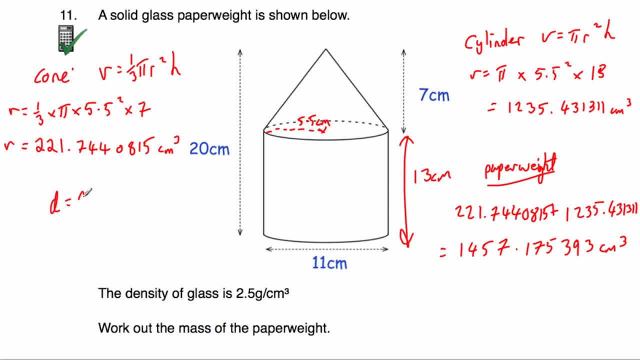 one way to do it. Another way to do it is to learn that density equals mass over volume. And if you find the mass, we're going to multiply both sides of the formula by volume. So multiply by volume and multiply by volume, So we're going to get density times. volume is equal to mass. So if we 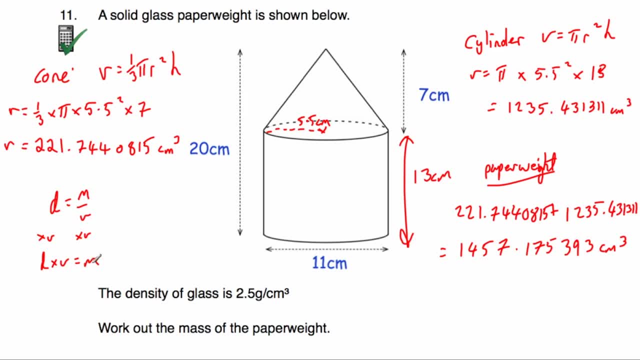 take the density 2.5 and multiply by volume, we'll get the mass. So that's another way to do it. Or another way some students do is to learn a triangle: density, mass and volume. And if you want to find mass, you cover it up. you do density times volume. Okay, but anyway, what we're going to do is we're 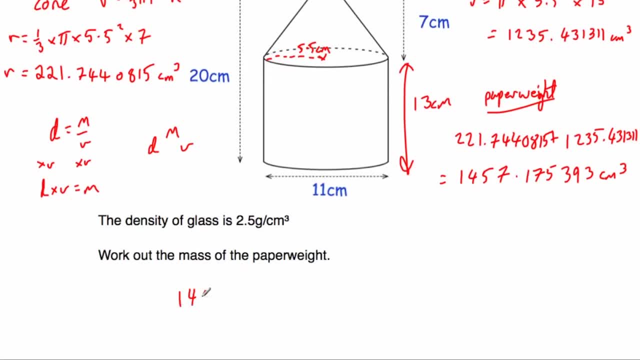 going to take the volume of the paperweight, which is 1457.175393.. And we're going to multiply that by 2.5, because each centimeter cubed has a mass of 2.5.. So we multiply the volume by 2.5, we'll get. 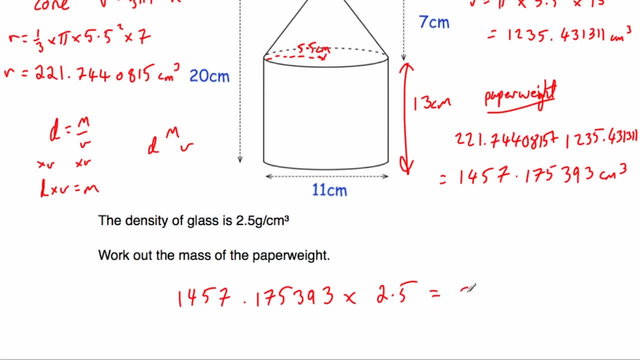 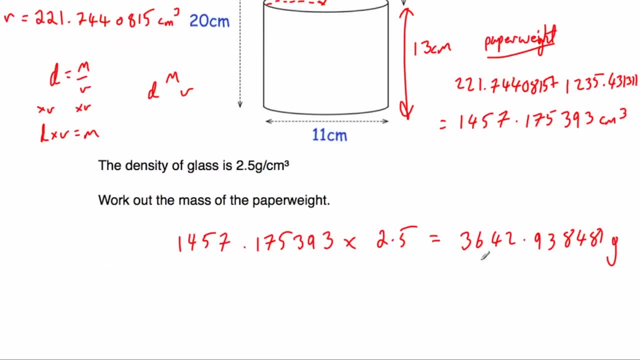 the mass of the whole thing. So multiply by 2.5 equals 3642.93848, and so on grams. So that's the mass of the paperweight in grams, And we could round it. We could round it to something such as: 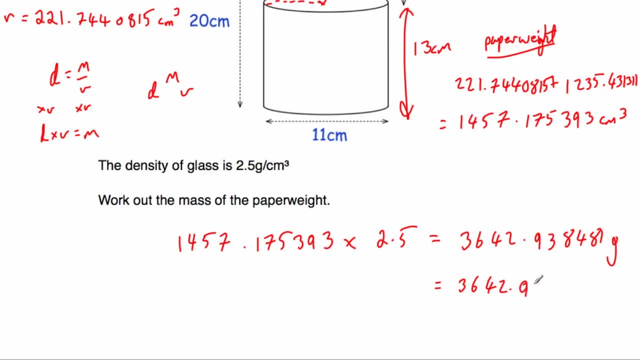 3642.94 grams. if we round it to two decimal places, We could even write it in kilograms. We could round it to 4.43.. We could round that kilograms and so on. So the answer is either 3642.94 grams. 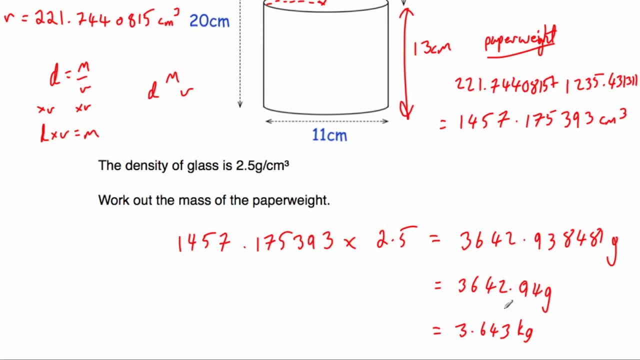 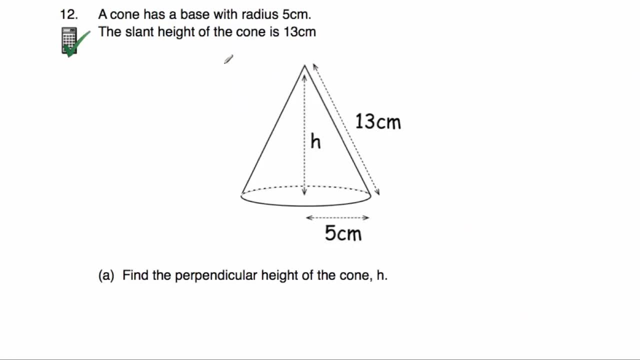 roughly, or 3.643 kilograms roughly. That's it. That's the mass of the paperweight. Okay, let's have a look at our next question. Okay, question number 12.. Question number 12.. We've got this cone and we're told the cone has got a base of radius 5 centimeters. So the radius of the base of the 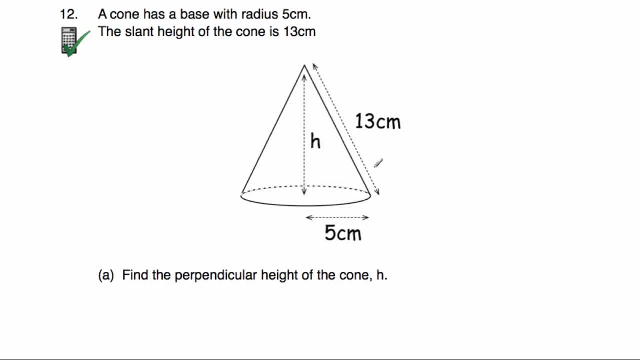 cone is 5 centimeters and the slant height of the cone is equal to 13 centimeters, And we've been told the height of the cone. Now, if you look at this, this is a right angle triangle where we have got the perpendicular height, We've got the radius and we've got the slant height, So we've got a 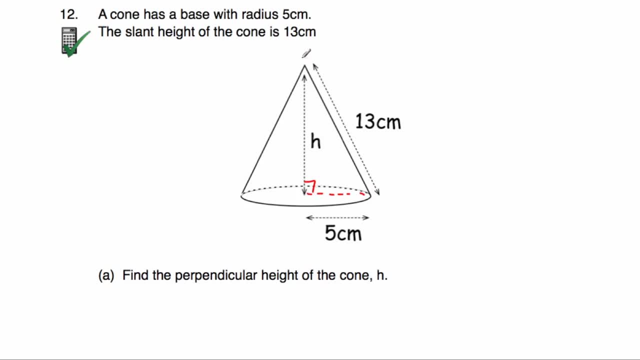 right angle here. We've got the shorter side of 5 centimeters. We've got the longest side is 13 centimeters. We want to find one of the other shorter sides, the height of the cone, And that is going to be Pythagoras's theorem. We're going to label the sides a, b and c. So I label a, the. 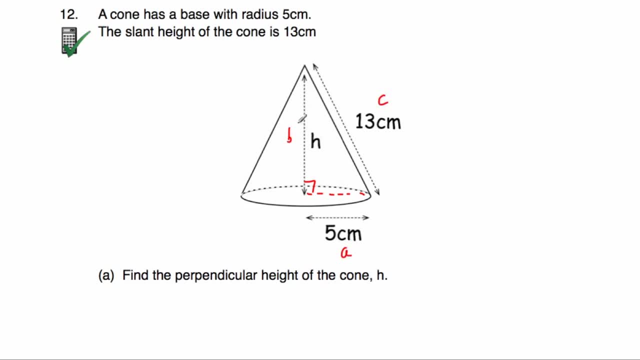 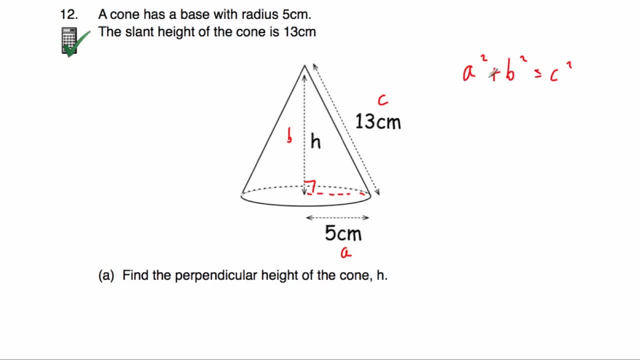 equals c squared. The two shorter sides squared added together will be equal to the longest side squared. So a squared, that's going to be 5 squared plus, and instead of b squared, that's going to be h squared And that is equal to c squared, which is 13 squared. 5 squared is equal to 25 plus h. 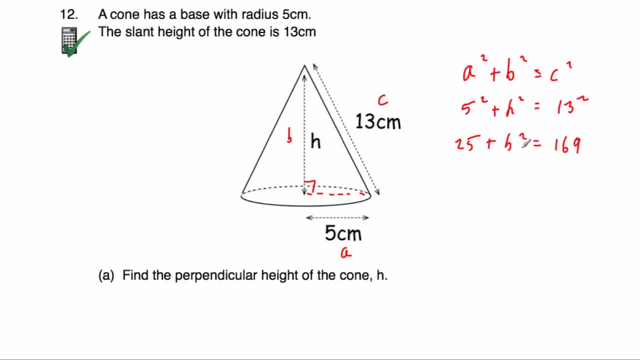 squared And 13 squared is equal to 169.. Then if we take away 25 from both sides, take away 25 and take away 25.. On the left hand side, we've got h squared that equals 144.. And then defined h, we're just going to square root. So we're going to square root 144. 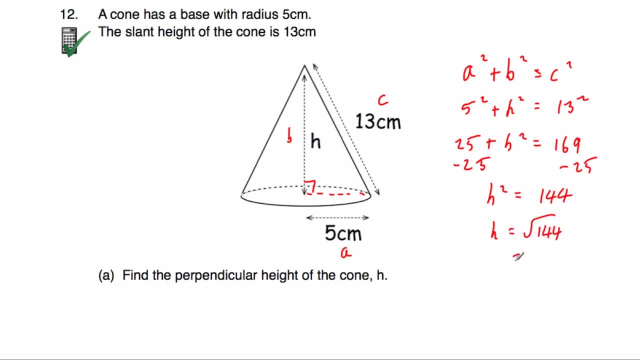 and the square root of 144 is equal to 12.. So the height of the cone is equal to 12 centimeters, and that's it. So the height of cone, the perpendicular height of the cone, is 12 centimeters, 12.. Okay, part. 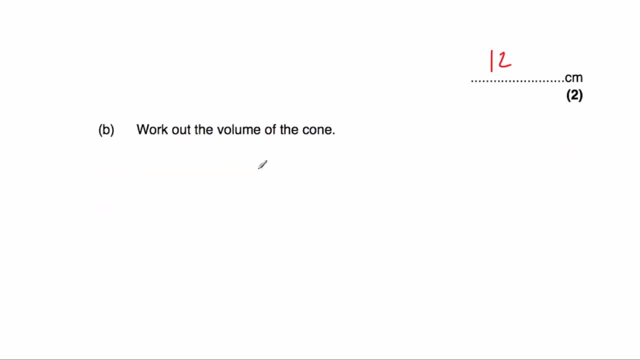 b, part b says: work out the volume of the cone. So the volume of the cone volume is equal to third pi r squared h. So we need to find the volume. So we need to know the radius and the height, So we know the height's 12.. 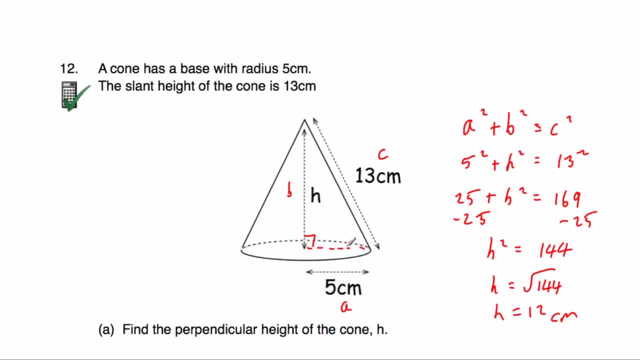 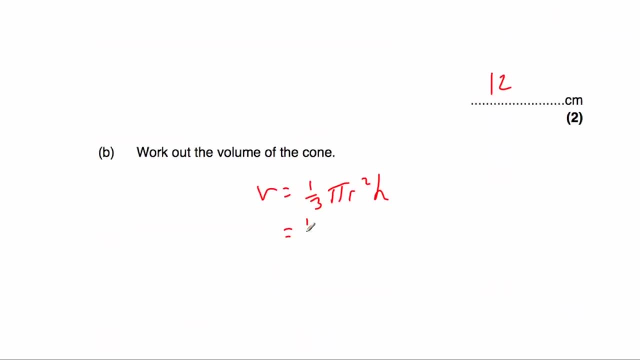 let's go up and get the radius. so we have a look: the radius of the cone is equal to 5, so the radius is equal to 5 and the height perpendicular height is equal to 12. so we go back down. here we've got that's equal to a third multiplied by pi, multiplied by the radius, which is 5, squared times by the. 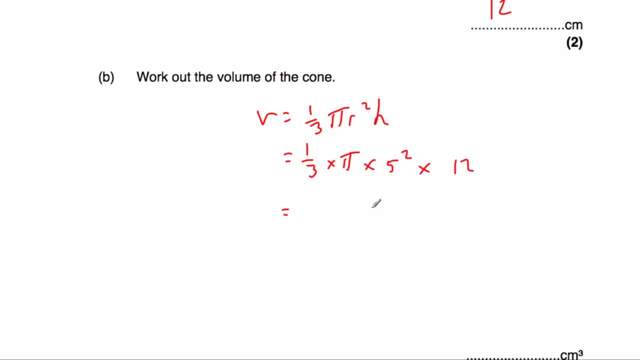 height, which is 12, and this is a calculator question, so we can just type this in. and when you type it in and press equals, we get that's equal to 100 pi, or as a decimal number that would be equal to 314.1592. and so on, centimetres cubed, and let's round our answer to two decimal places. 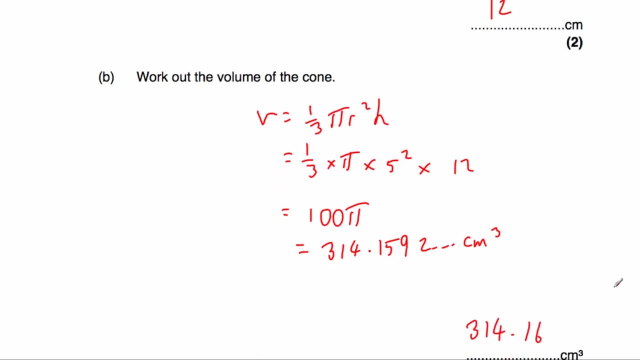 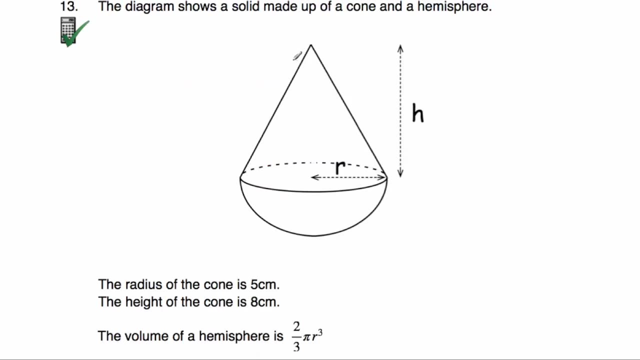 answer would be 314.16 centimetres cubed, and that's it. that's the volume of that cone. okay, let's have a look at our next question. okay, let's have a look at question number 13. so question number 13 says the diagram shows a solid made up of a cone. so we've got this cone and a hemisphere. 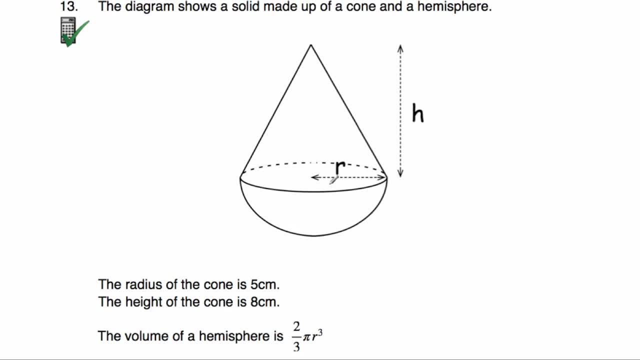 so half a sphere, and that's the base of it and we're told the radius of the cone is five centimetres. so the radius of the cone is five centimetres and the height of the cone. the height of the cone is eight centimeters and we're told the volume of a 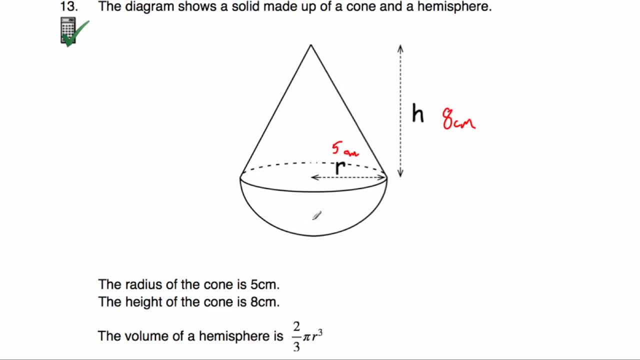 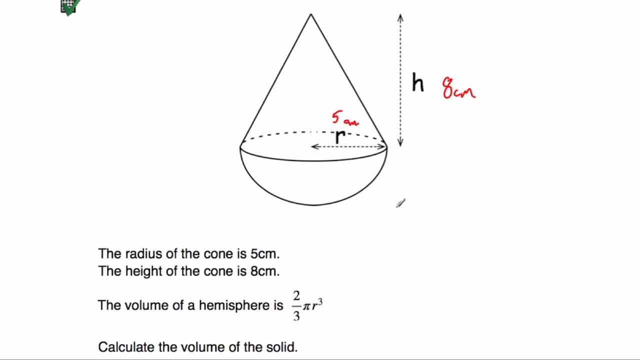 hemisphere is two-thirds pi r cubed. so to find the volume of this hemisphere, we're going to do two-thirds pi r cubed and the question says: work out or calculate the volume of the solid. so we need to find the volume of this shape. so let's start off with the cone. so if the cone, the volume. 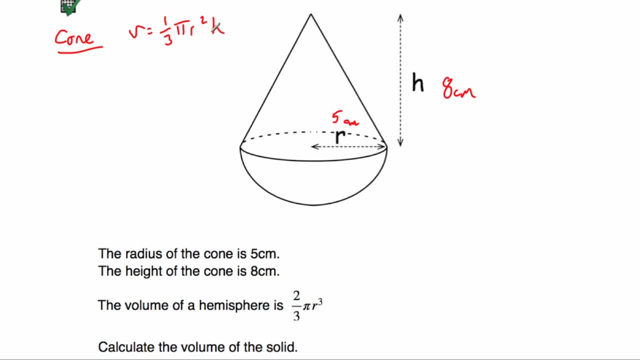 is equal to a third pi r squared h. so the radius of the cone is equal to five and the height of the cone is equal to eight. so the volume will be equal to a third multiplied by pi, multiplied by the radius, which is five squared, multiplied by the height, which is equal to eight. so when we type that, 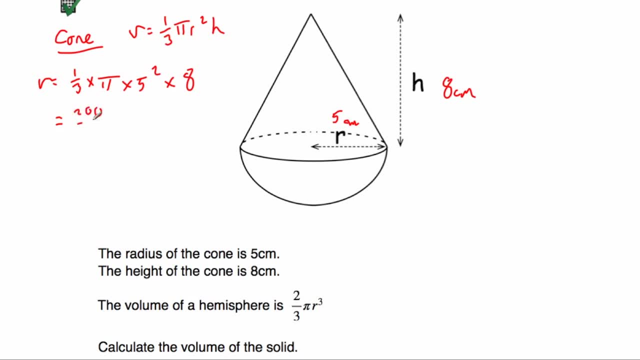 into our calculator and when we press equals we get an answer of 200 over three pi centimeters cubed, or we could write it as a decimal, which would be equal to 209.4395102 centimeters cubed. so that's the volume of the cone and, in terms of the hemisphere, the volume of the hemisphere. 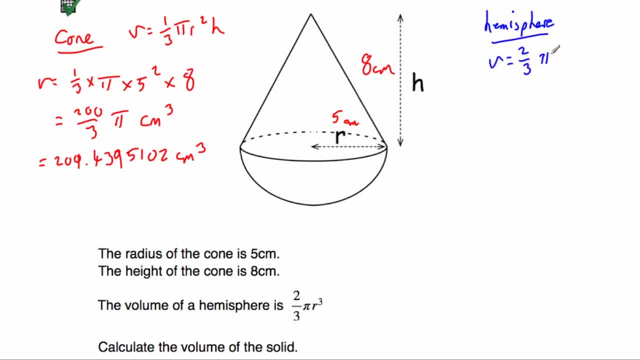 is equal to. the volume is equal to two-thirds pi r cubed. so we just need to find the radius of the hemisphere. now, if you look at it, the radius of the cone would also be the radius of the hemisphere, and that's equal to five centimeters. so that means that the volume would be equal to. 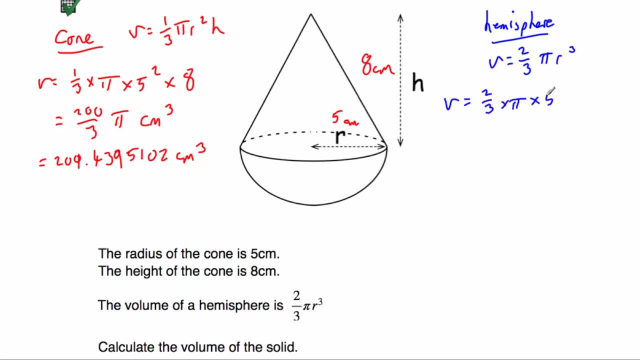 two-thirds multiplied by pi, multiplied by five cubed, and when we do that we get that's equal to 250 over three pi centimeters cubed, or as a decimal number it would be 261.79. three eight, seven, eight centimeters cubed. so that's the volume of the cone and that's the. 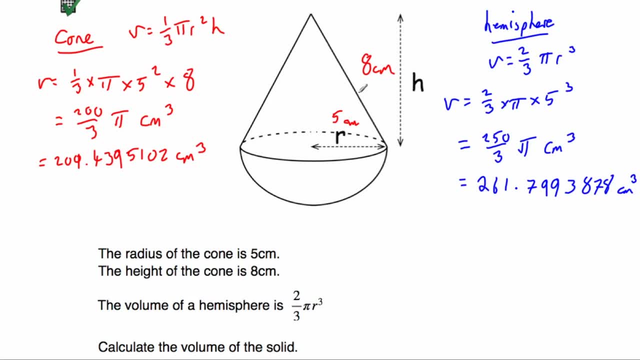 volume of the hemisphere and if we just add them together we'll get the volume of the solid, and you can either do 200 over three pi plus 250 over three pi and get that answer. alternatively, you could add these two numbers together and both of them will work, and when you add them together we 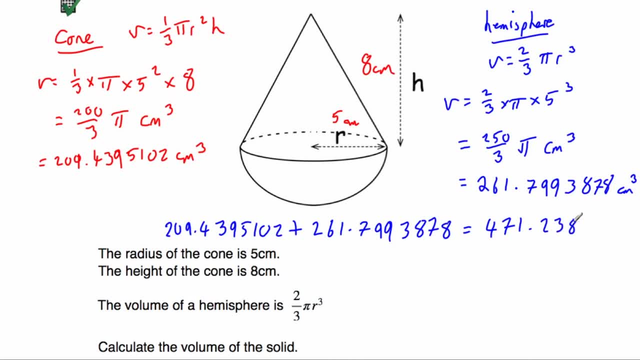 get an answer of 471.238898 centimeters cubed and we could round that. let's just round it to one decimal place. that'll be 471.2398 centimeters cubed. so that's one way we could do it. alternatively, we could have added together the: 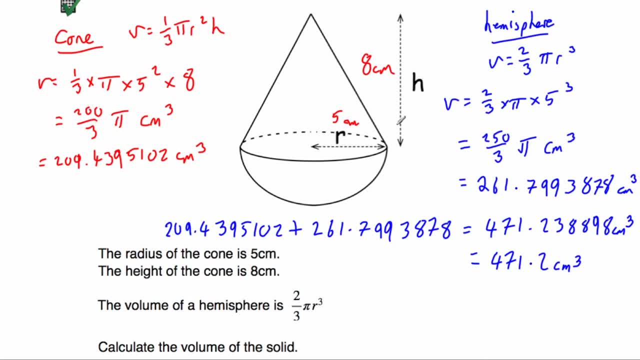 200 over 3 pi and the 250 over 3 pi. so let's do that, and that's equal to 150 pi, which is quite nice, and then whenever we convert that to decimal, we also get that's equal to 471.2 centimeters. 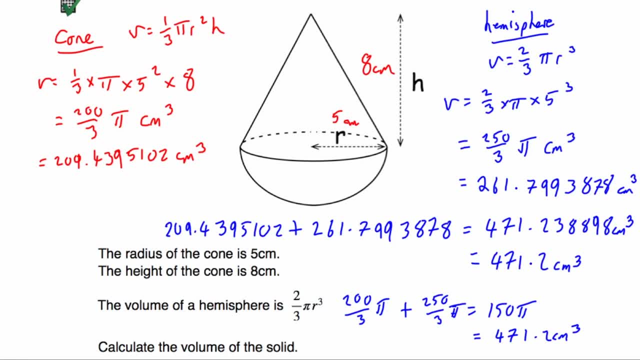 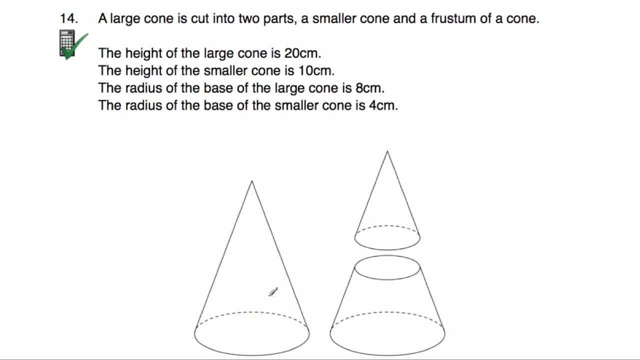 cubed to one decimal place and that's it. so that's how you find the volume of that solid. okay, let's have a look at our next question. okay, let's have a look at question number 14. so question number 14 is a large cone. so this large cone on the left hand side is cut into two parts. a smaller cone- 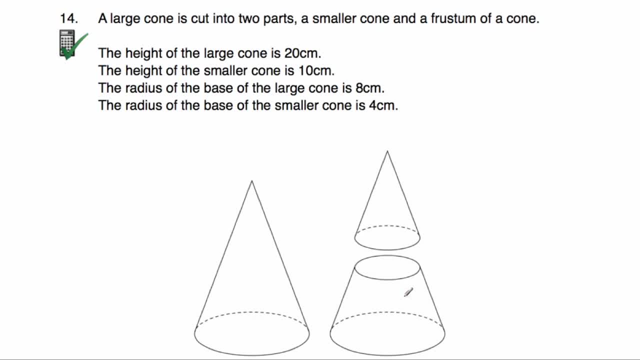 so this part and a frustum of a cone. so a frustum is just what you've got left when you chop the top of a cone off or a top of a pyramid off or things like that. so this is a frustum of a cone. so this: 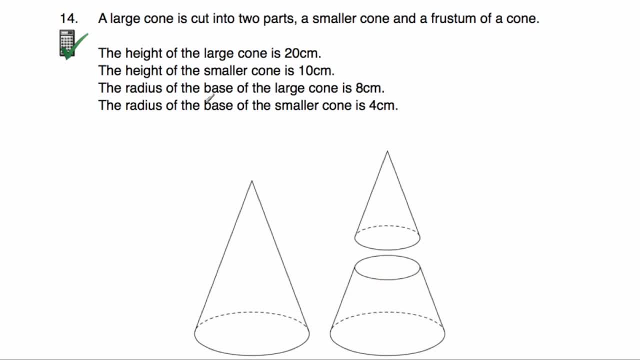 bottom bit's what you've got left whenever you chop the top of the cone off, and the height of the large cone is 20 centimeters, so the height of the large cone is equal to 20 centimeters, so that's 20 centimeters, and the height of the smaller cone is 10 centimeters, so that's got a height of 10. 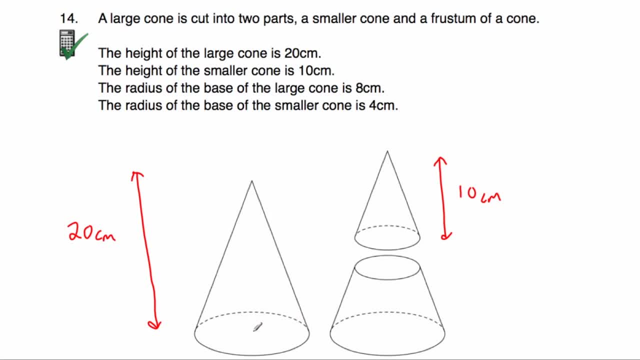 centimeters and the radius of the base of the large cone. so the radius of the base of the large cone is equal to 20 centimeters. so that's 20 centimeters and the radius of the base of the large cone is to eight centimeters and the radius of the base of the smaller cone is equal to four centimeters. 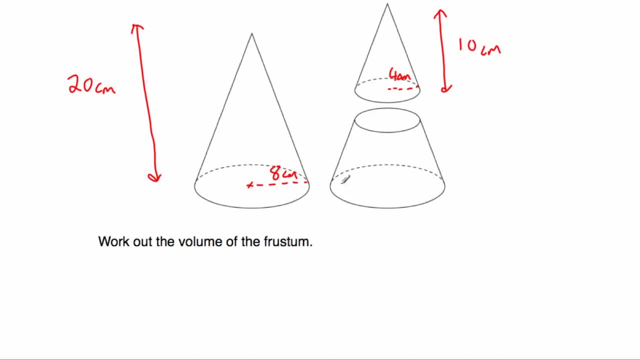 and the question asked is to work out the volume of the frustum. so we've been asked to work out the volume of this frustum. so to do that, what i'm going to do is: i'm going to work out the volume of the larger cone, i'm going to work out the volume of the smaller cone and if we take the 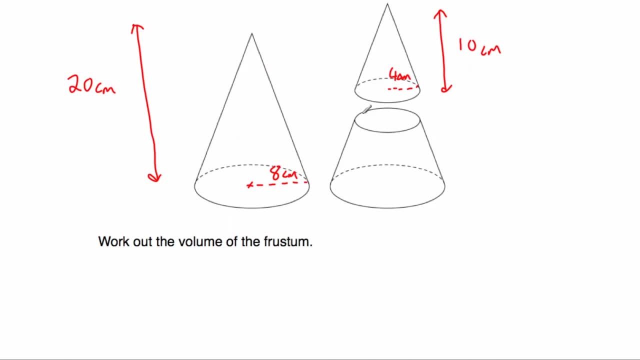 volume of the smaller cone. away from the volume of the bigger cone, what's left would be the volume of the frustum. so let's do that. let's find the volume of the larger cone to begin with. so the larger cone, the volume is equal to third pi r squared h. so it's going to be equal to a third. 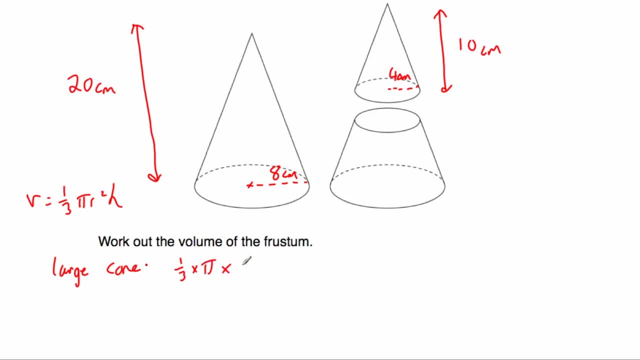 multiplied by pi, multiplied by the radius squared, so it's going to be eight squared multiplied by the height, which is 20, and when we do that- and it's a calculator question- we get that's equal to 1280 over 3 pi, or 1340.412866 centimeters cubed. so that's the volume of the. 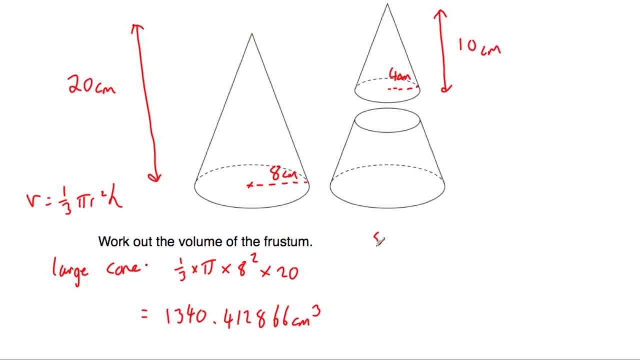 larger cone. now if we work out the volume of the smaller cone, so the small cone, small cone, that's equal to a third multiplied by pi, multiplied by the radius squared, so it's going to be four squared times by the height 10, and when we do that we get that's equal to 160. 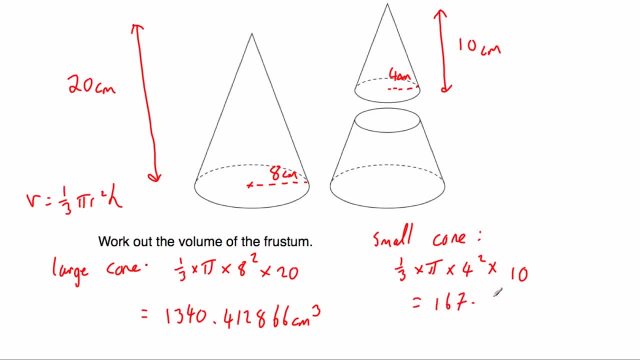 over 3 pi, or 167.5516082 centimeters cubed. and so if we take the volume of the small cone away from the volume of the large cone, we'll be left with the volume 167.5516082 centimeters cubed. and so if we take the volume of the small cone away from the volume 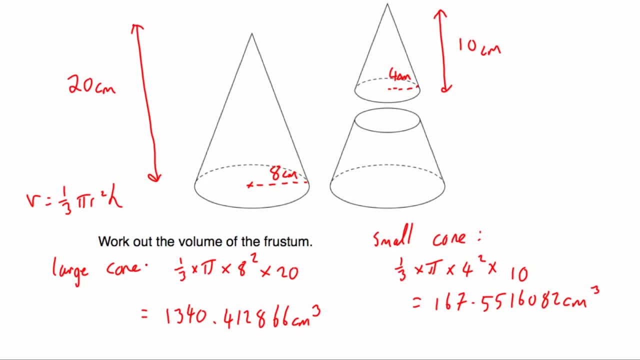 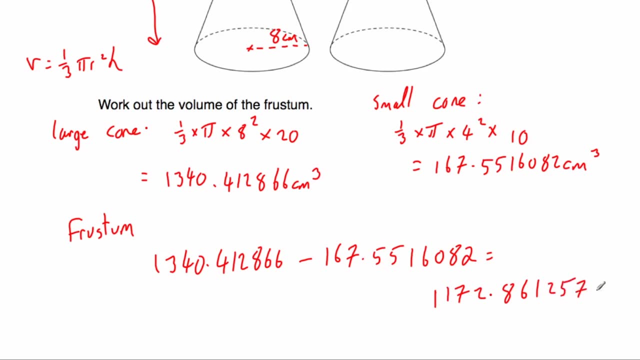 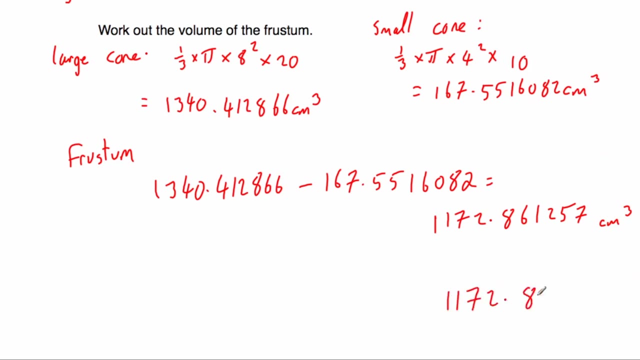 of the frustum. so we just need to take this away from this. so let's do that, and when we do that we get an answer of 1172.861257 centimeters cubed and we could round that. let's round it to two decimal places. that'll be 1172.86 centimeters cubed and that's the volume of the frustum. and 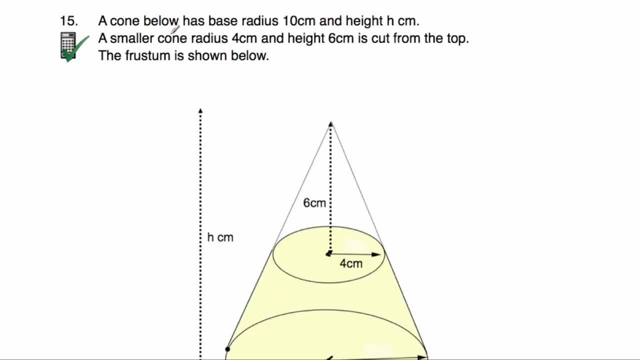 that's it okay. let's have a look at question number 15. so question number 15 says the cone below has got a base radius of 10 centimeters and a height of 8 centimeters and a small cone of radius 4 centimeters and height 6 centimeters is cut from the top and the frustrum is shown below. 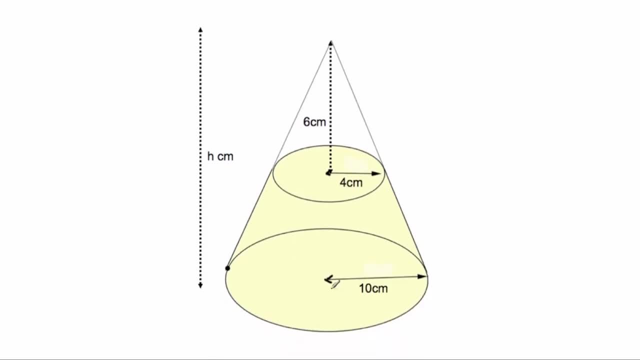 so let's have a look and see what we've got. so we've got the large cone that's got a base radius of 10 centimeters and a height of 8 centimeters, and in yellow we can see the frustum that's left after the cone on the top has been chopped off, and the cone on the top would have had a radius. 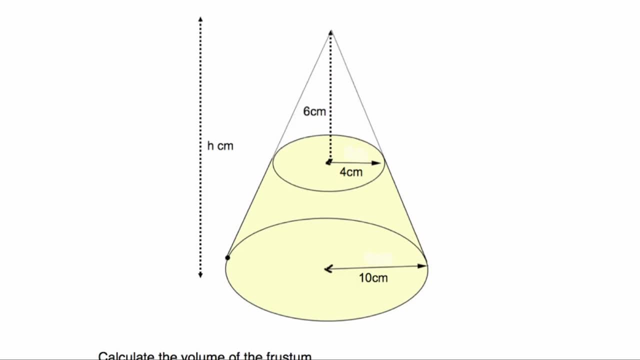 of 4 centimeters and a height of 6 centimeters, and the question asks us to work out the volume of the frustrum. so, again, what we're going to do is we're going to work out the volume of the large cone. we're then going to work out the volume of the small cone. 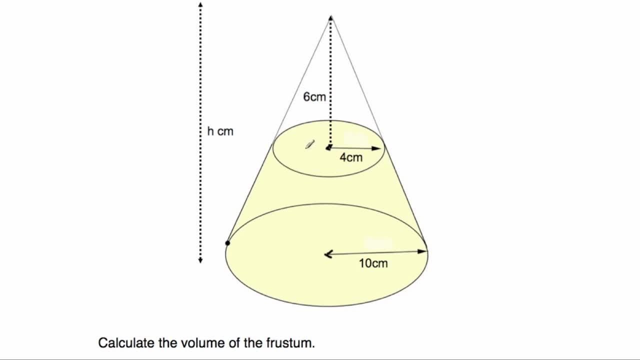 cone that's been removed and then take it away to see what's left of the volume of the frustrum. Now, if we have a look here, we can work out the volume of the small cone quite easily, because we've got a radius of four and a height of six. but when we look at the large cone it's got a. 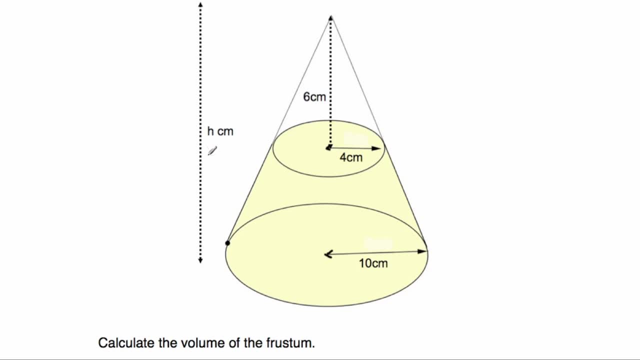 radius of 10 centimetres, but the height we don't know. but we need to find the height to be able to work out its volume. Now, whenever we're dealing with frustrums and we're chopping off cones from the top of larger cones, the two cones are mathematically similar. What that means is: 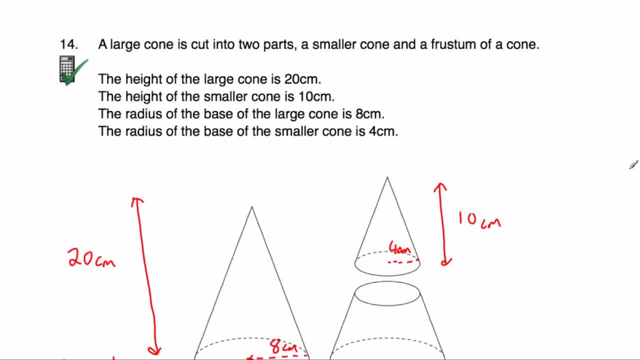 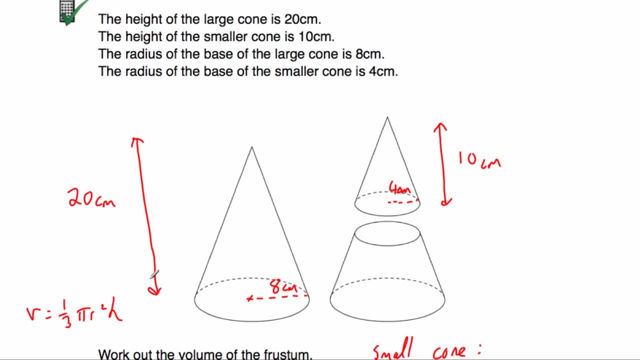 they're enlargements of each other. If we look at the previous question, we look at this question, here we had the two cones. one has got a radius of four and a height of 10 and the other has got a radius of eight and a height of 20.. So if you look at it, you've doubled the lengths, the length of the. 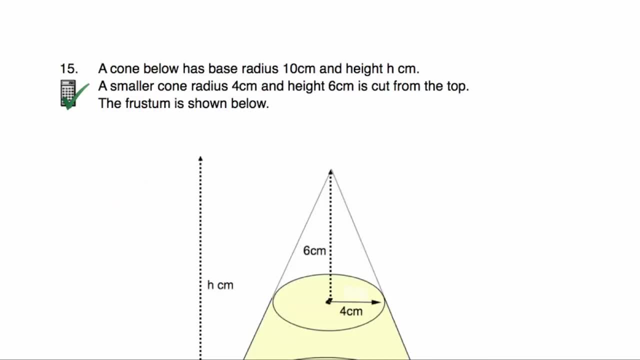 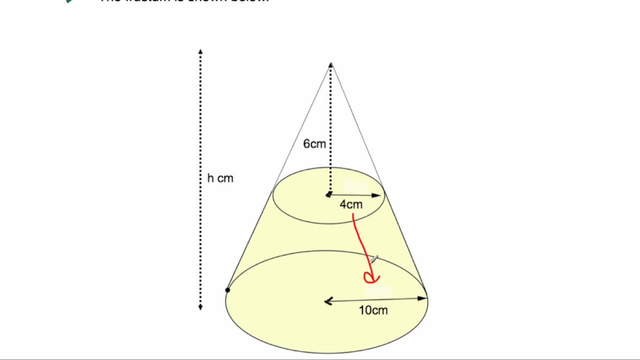 radius has been doubled and the height has been doubled. So if we have a look at this cone here, we have got the radius of the smaller one and we've got the radius of the larger one. So if we divide 10 by 4, we can see what we would multiply by. we can see how many times larger 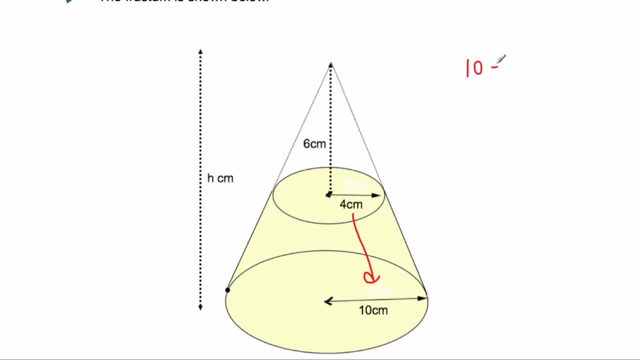 the larger cone is than the smaller cone. So if we do 10 divided by 4, that's equal to 2.5.. So that means we've got a radius of 4 and a height of 10.. So if we look at the previous question, 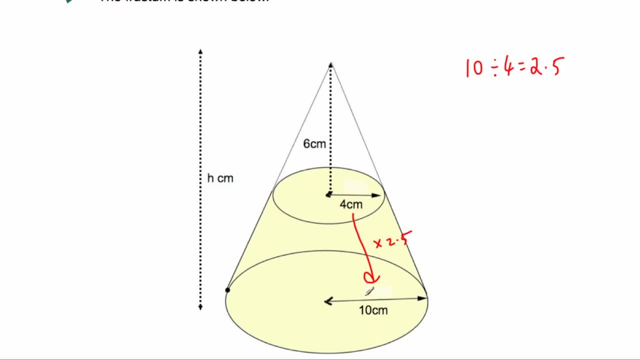 we can see that this radius is 2.5 times bigger than this radius and that means the height of the larger cone will be 2.5 times bigger than the height of the smaller cone. So if I multiply by 2.5, so multiply by 2.5, that will give me the height of this larger cone. So whenever we do 6 times 2.5, 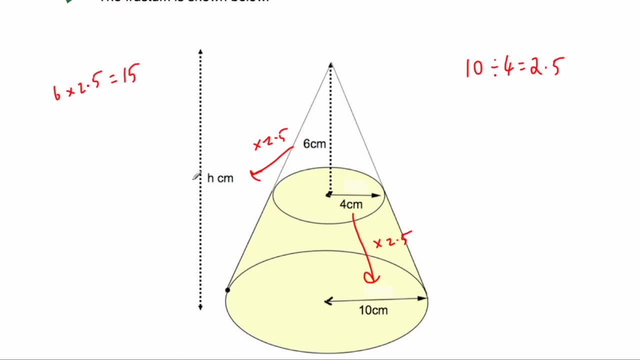 so 6 times 2.5 that's equal to 15 centimeters. So that means the height of the larger cone will be 15 centimeters, and that's great because now we know the radius of the larger cone and the height of the larger cone, we can work out its volume. 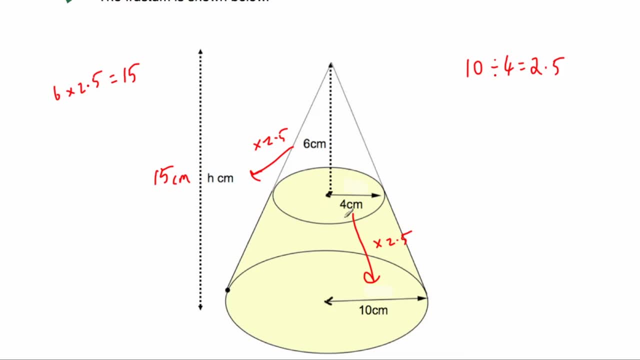 We can work out the volume of the smaller cone and take them away to see what's left for the volume of the frustum. So let's do that. So for the large cone we've got the volume. So the volume is equal to a third pi r squared h, So that for the large cone the volume would be equal to a third multiplied. 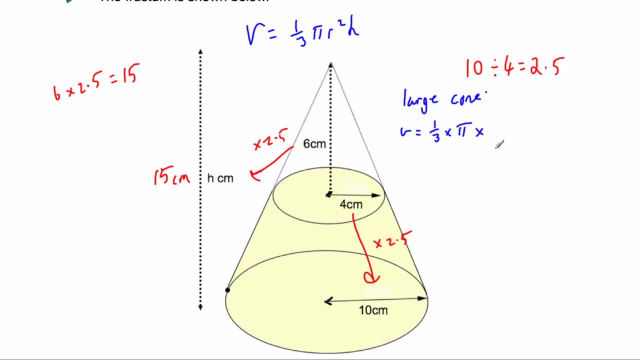 by pi, multiplied by the radius squared. So the radius of the large cone is 10, so times by 10, squared times by the height, which is 15.. And when we do that, we get an answer of 500 pi or 1570 point 796327 centimeters cubed. So that's the volume of the large cone In terms of the smaller cone. 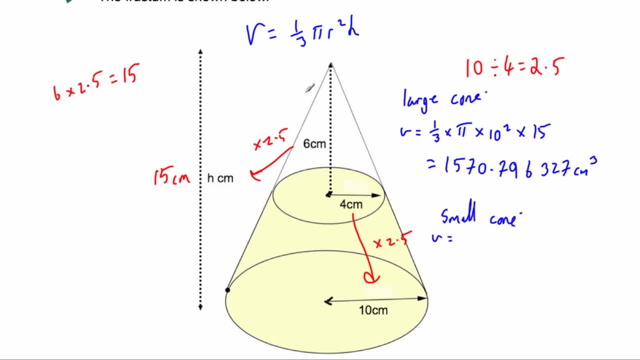 the small cone. Now, in terms of the small cone, its volume is going to be equal to. if we have a look at the small cone, it's going to be a third multiplied by pi, multiplied by the radius squared. So it's going to be 4 squared multiplied by its height, which is 6.. And when we do that, we get that's. 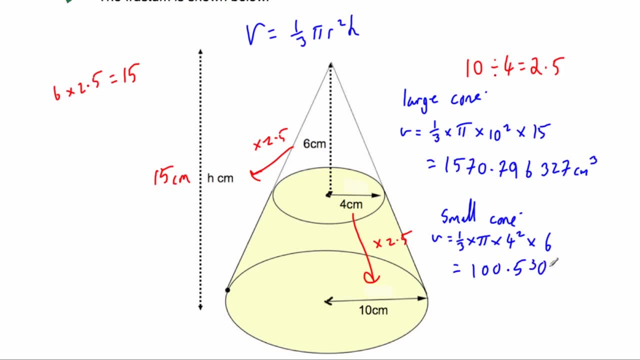 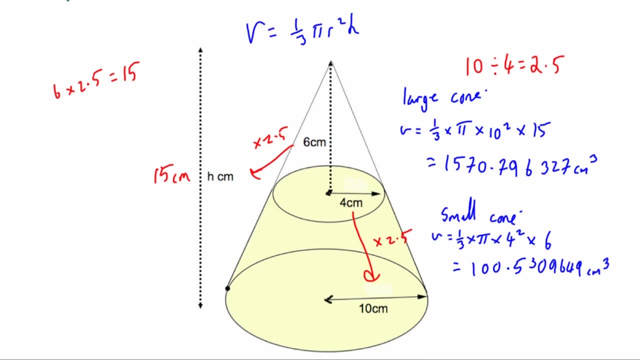 equal to 32 pi or 100, point 5309649 and so on, centimeters cubed, And then, if we take them away, we can then find the volume of the frustum. So let's do that, And when we do that we get an answer. 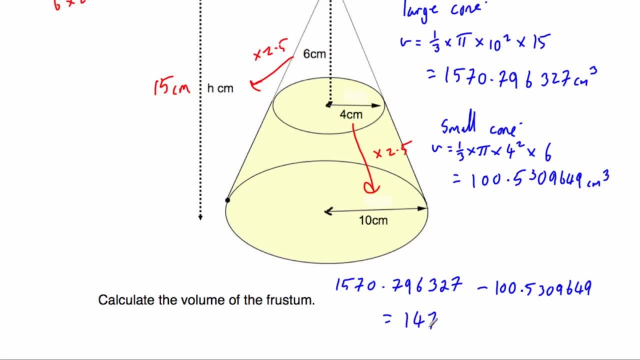 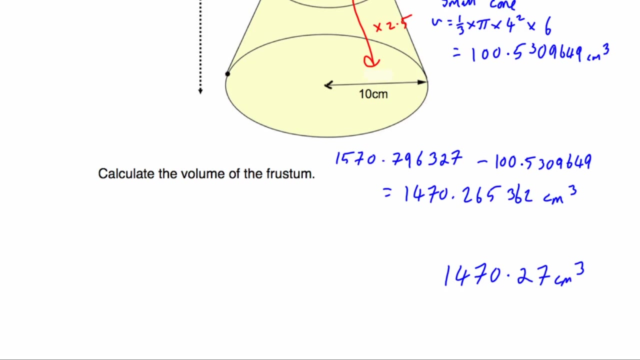 of 468 pi or 1470 point 265362 centimeters cubed, And that's the volume of the frustum. And the answer is- and let's round it to the decimal place- is 1470 point 27 centimeters cubed. Okay, let's. 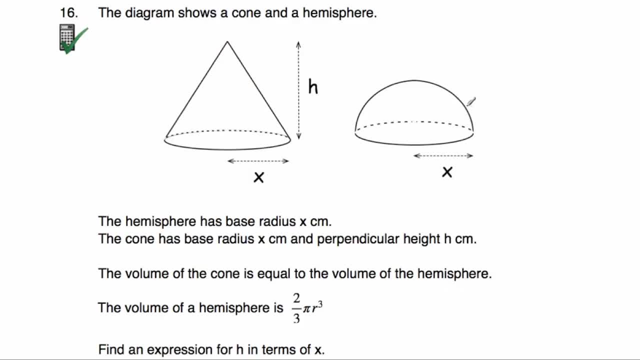 have a look at our next question, So question number 16. we've got a cone in a hemisphere and we've got their dimensions. the radius of the cone is equal to x, the height of the cone is equal to h and in terms of the hemisphere it's got a radius of x as well. And we're told the 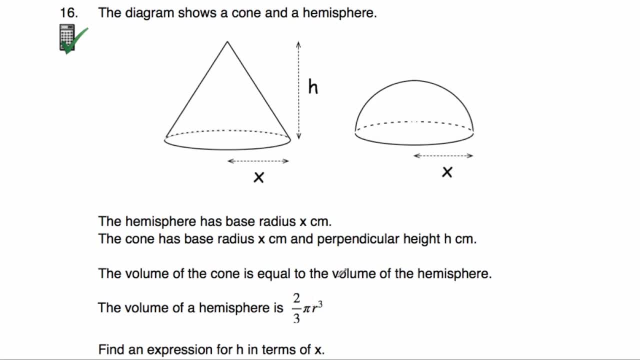 volume of the cone is equal to the volume of the hemisphere, And we've been given the formula to find the volume of the hemisphere, which is two thirds pi r cubed, And we've been asked to find an expression for h in terms of x. So, in this case, what I'm going to do is I'm going to find: 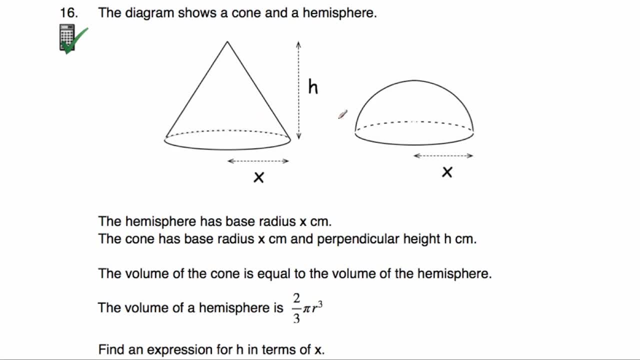 the volume of the cone and I'm going to find the volume of the hemisphere in terms of x and h, And then we're going to put them equal to each other and see what we can do. So let's start off with the cone. So, with the cone, its volume is equal to the volume is equal to the volume of. 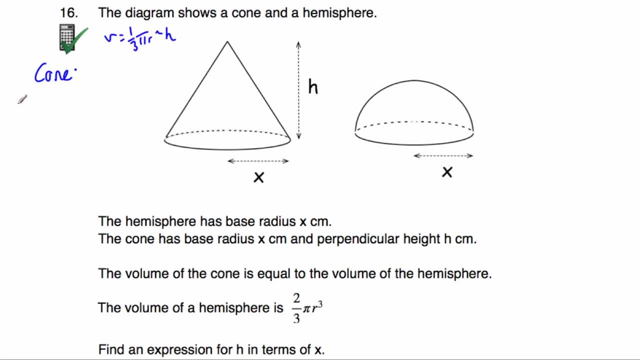 third pi r squared h, so it's going to be the volume is equal to a third multiplied by pi, multiplied by the radius squared, so it's going to be x squared. so times by x squared multiplied by the height, which is h, so the volume of the cone would be a third pi x squared h. so that's the. 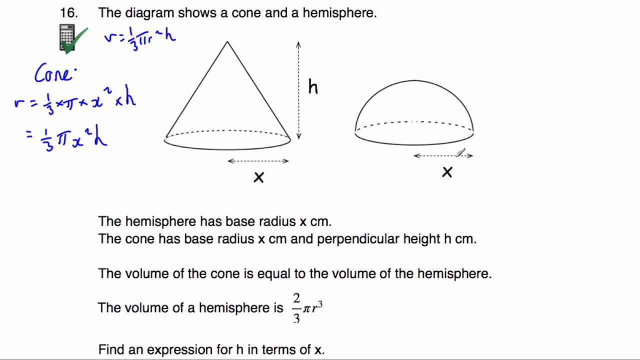 volume of the cone. now let's look at the hemisphere. well, with the hemisphere, the radius is equal to x, so the volume would be equal to two thirds pi x cubed. so just replacing the radius with x. now we're going to put them equal to each other. so let's put those two equal to each other and see. 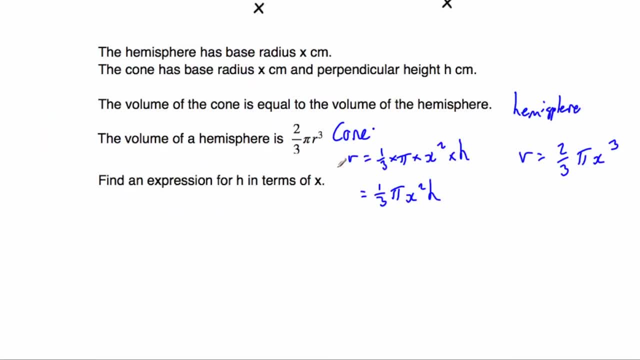 what we get. so let's just bring it down here and down here. so here we've got the volume of the cone and here we've got the volume of the hemisphere. now we're told that they're equal to each other. so let's write that down: a third pi x squared h is equal to two thirds pi x cubed. and we want to. 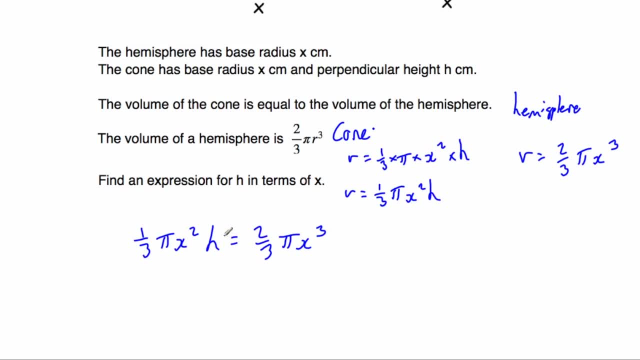 find that expression for h in terms of x. that means we want to make h the subject. so let's try and make h the subject. that means we want to get h on its own. so let's start off by dividing both sides of this equation by pi. if we divide by pi and divide by pi, that will get rid. 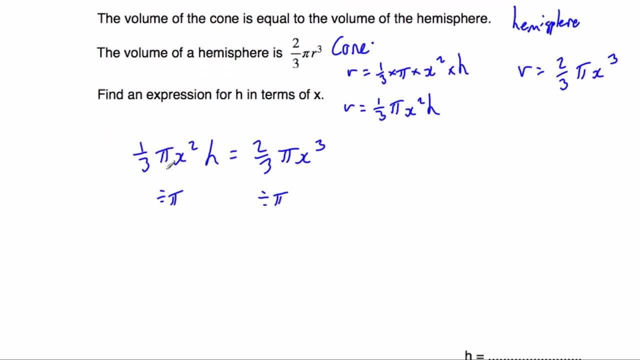 of the pi's. so i'll just make that a little bit easier. that's how we give us. on the left hand side we're dividing by pi to get rid of this pi, so that'll leave us with a third x squared h, and on the right hand side that would leave us with two thirds x cubed. now we want the h on its own, so 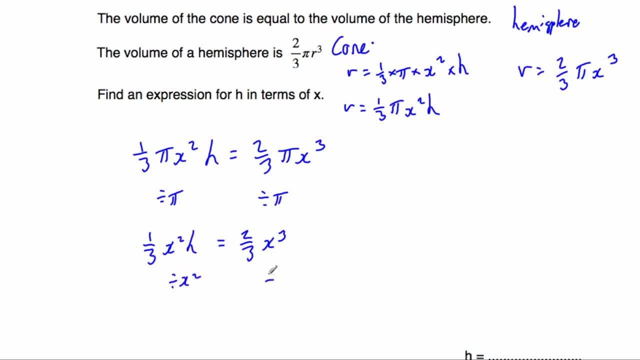 let's get rid of this x squared. so let's divide by x squared and divide by x squared, so that's going to be: on the left hand side we'll be left with a third h, and on the right hand side we had two thirds x cubed. we're. 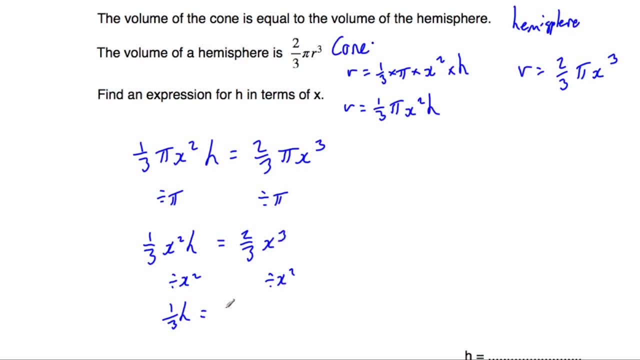 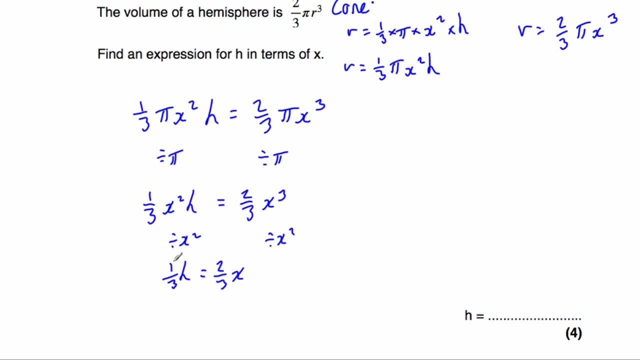 divided by x squared. when we divide x cubed by x squared, we're just left with x. so we'll get two thirds x. so we're nearly there. we've got a third. h is equal to two thirds x. now we don't want this third here. now we can get rid of this third in a couple of ways. we could divide both sides of the. 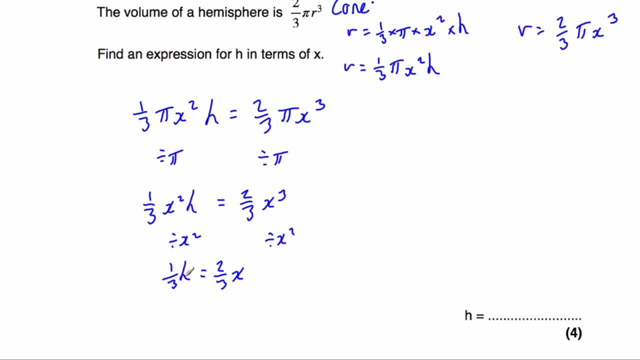 equation by a third, because this is a third times h and to get rid of that we could divide both sides by a third. and if we do, two thirds divided by one third, we could get our answer that way. i, personally, in this question, what i would do is i would just times both sides by three, because if 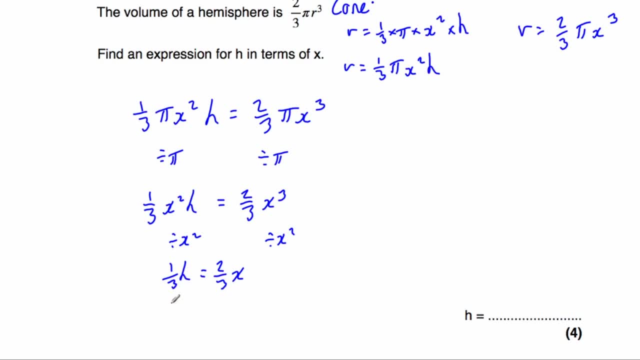 we have got a third of something. we're to find that something that h i would just times by three and times by three. so a third of h times three, that'll just be h. and then we've got two thirds x times three. so we need to do two thirds times three, so two thirds multiplied by three, which is 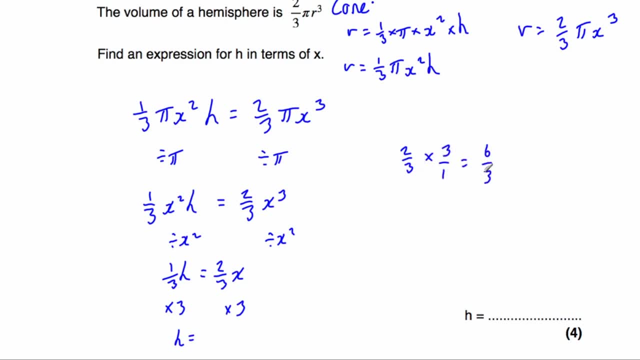 three over one. two times three is equal to six, and three times one is equal to three. six divided by three is equal to two, so that would be two x. so h equals two x, and that's it. so h is equal to two x. okay, let's have a look at our last question, so question number 17. we have got this sector. 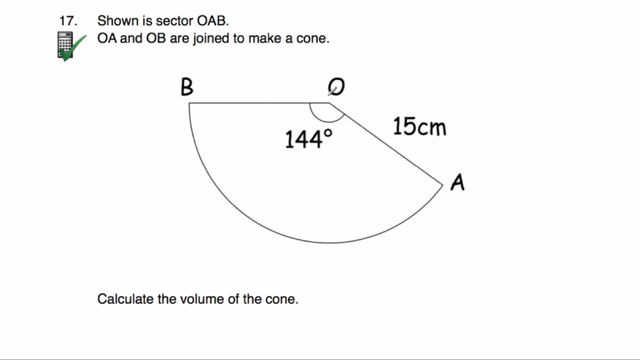 and it's the sector o a, b and the lines o a and o b are joined together to make a cone. so we're going to make a cone. let's do a sketch of that cone so it would look something like this. so our cone would look something like that and in terms of our cone, we've got the slant height we know. 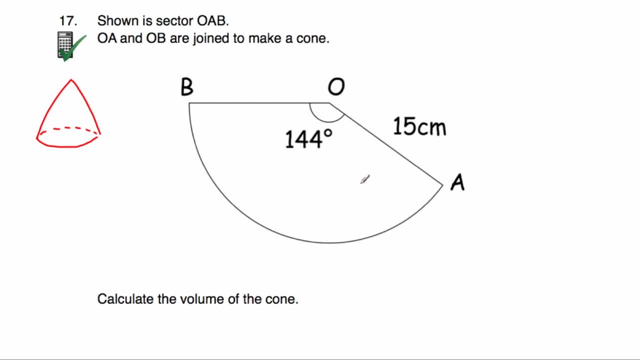 that that's going to be equal to 15, because whenever we join that up, that sector, and join up the o a and the o b, those two lines are going to join together to be over here somewhere. so that would be the slant height 15.. 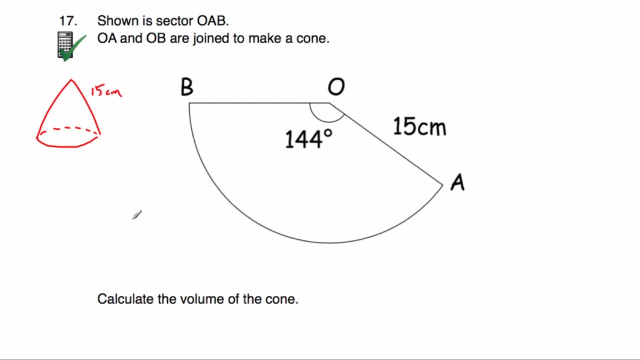 centimeters and in this question we've been asked to work out the volume of the cone. so we want to find two things: we want to find the radius of this cone. we want to find the radius of it and we want to find the perpendicular height of it. so the height of it and if we can find the 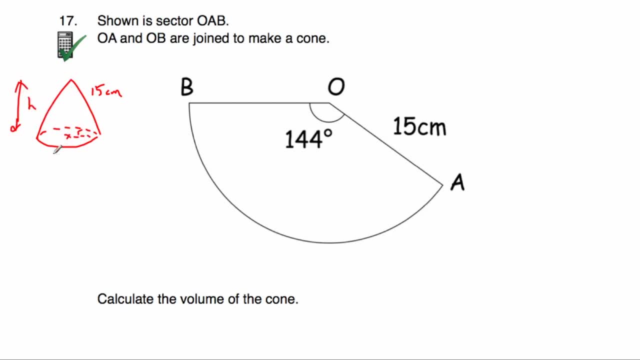 radius r and the height of it, h, then we can find the volume of the cone. now we're actually given some more information. we told this angle 144 degrees. so what we can do is if we consider, remember, if we go back to our topic, arc length, if we can work out the length of this arc a, b. 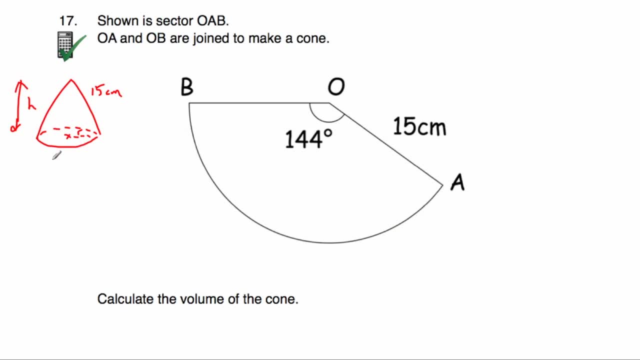 the length of this arc. a, b will be the circumference of the circle, and if we can find the circumference of the circle, we can then find the diameter of the circle and then, if we half that, we'll get the radius of the circle. so that's going to be really. 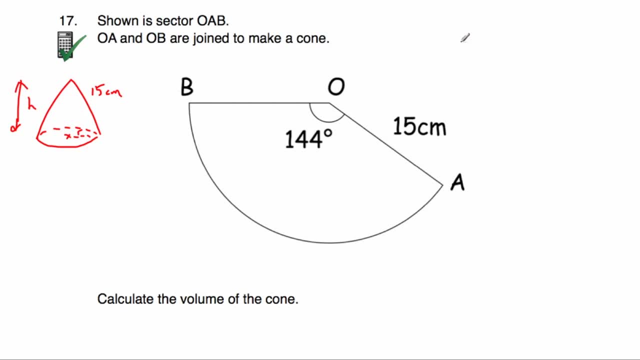 useful. so let's find the length of this arc a b. so the length of arc a b is going to be equal to veta over 360 times pi, times by the diameter. so veta is the angle which is equal to 144 divided by 360, because it's 144: 360 of a full circle, times by pi and times by the diameter of the. 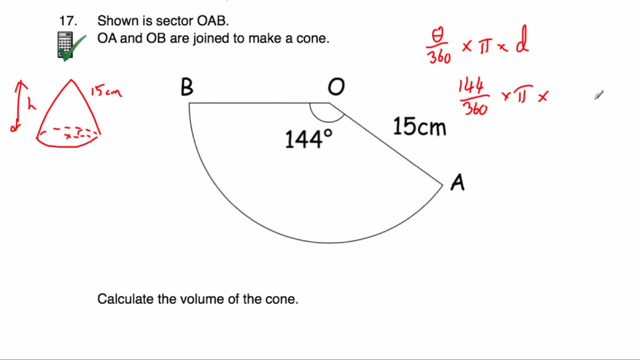 whole circle. now the diameter of this whole circle would be equal to 30 centimeters. so we're going to times by 30.. so whenever we do 144, 360 times pi, times 30, we will get the arc length a, b, and whenever we do that we get that's equal to 12 pi. 12 pi or 37.69911184 centimeters. 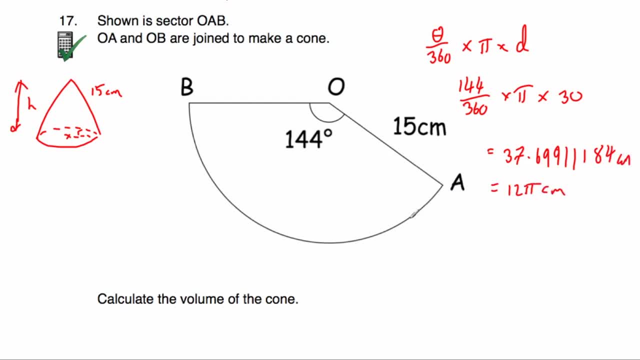 or 12 pi centimeters. so that means the arcline from a to b will be 12 pi centimeters. so 12 pi centimeters would be from a round to b or 37.69911184 centimeters, and that's the arcline. 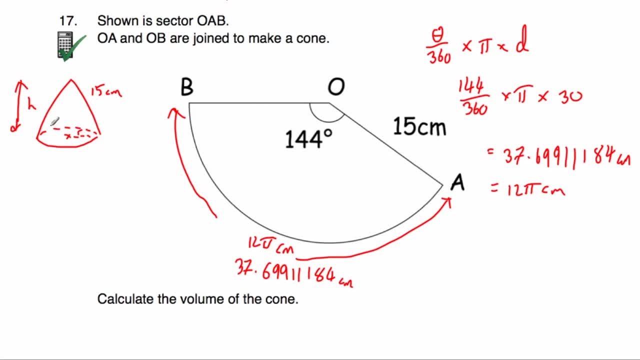 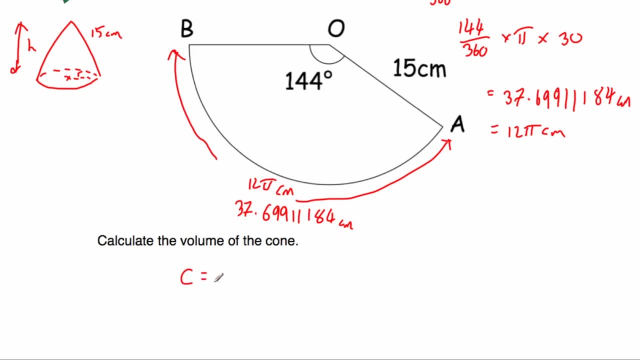 so whenever we join oa and ob together, that then will become the circumference of the circle on the base of the code. so that's the circumference of the circle. so remember, with circumference we've got circumference equals pi times diameter. so we've got circumference equals pi times diameter. 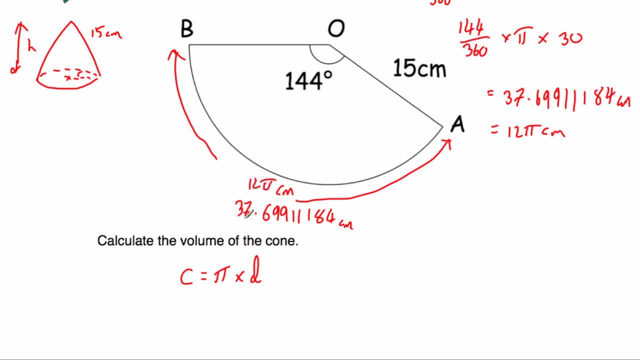 so we've got the of the circle. that's either equal to 12 pi or 37.699, and so on. we could use either one of them. i'm going to use 12 pi, and that's equal to pi times diameter. well, if we divide both sides by, 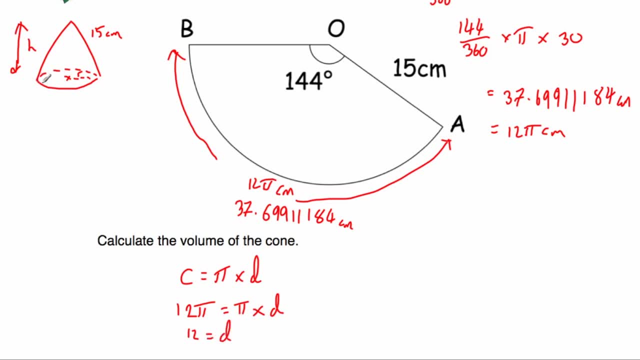 pi here we're going to get. the 12 equals the diameter, so the diameter of this circle is equal to 12, and then, if we half it, that means the radius is equal to 6. now we need to just find one more thing, and that's the perpendicular height of the cone. now, if you have a look at it, here we've got. 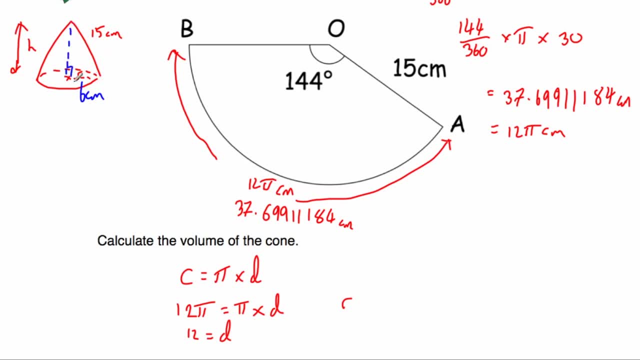 a right angle triangle. we've got this right angle triangle. we've got one of the shorter sides of the right angle triangle, being six centimeters. there's another shorter side, which is the h, which we're trying to find, and we've got the longest side, the hypotenuse, which is the slant. 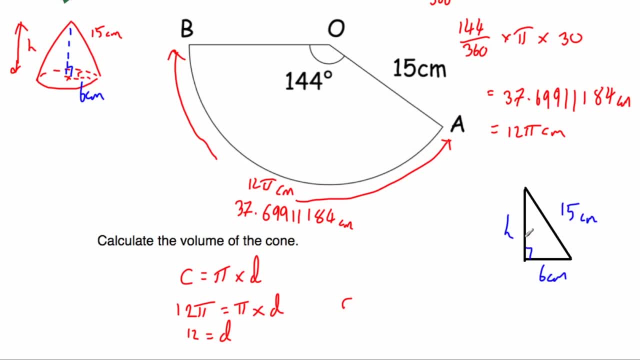 height, which is equal to 15 centimeters. so let's actually sketch that. so here i've just done a sketch where we've got our radius of six centimeters, we've got our slant height of 15 centimeters and we've got the perpendicular height. so let's use pythagoras's theorem. so let's label. 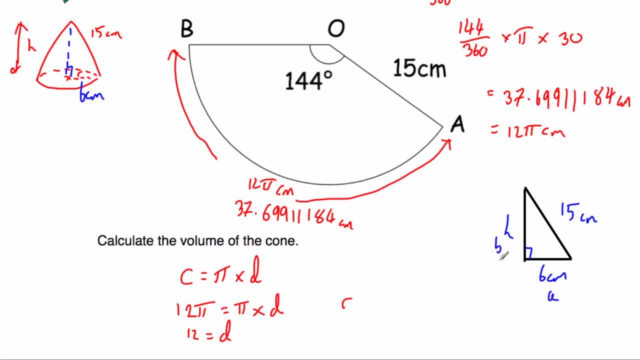 our sides a, b and c. so the two shorter ones, a and b. and remember, it doesn't actually matter which way around you label those, but the longest one will have to be c. so we've got the hypotenuse of c. so we've got a. 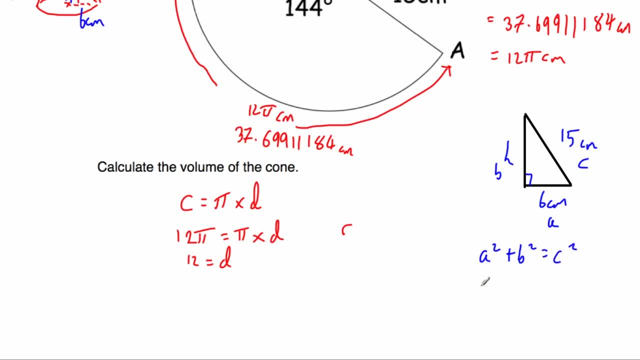 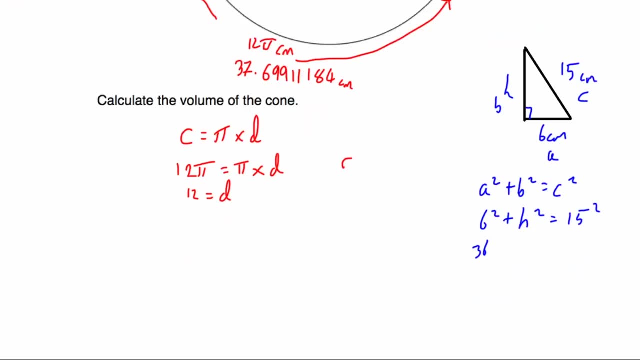 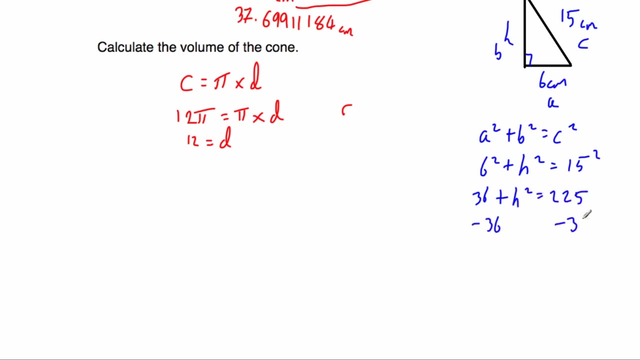 a squared plus b squared equals c squared, so it's going to be 6 squared plus h squared is equal to 15 squared. 6 squared is 36- let's just go scroll down here- plus h squared is equal to 225. if we take away 36 and take away 36, we get the h squared is equal to 225. take away 36 is equal to 189 and 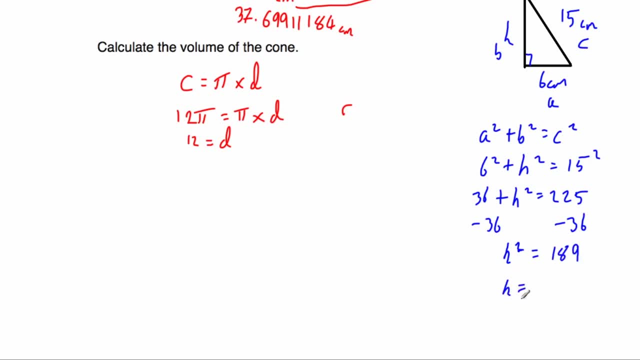 whenever we square root that we get the h is equal to the square root of 189, which is equal to 3 root 21 or 13.74772708 centimeters. so we've got the. if we go back up to our cone, we have got. 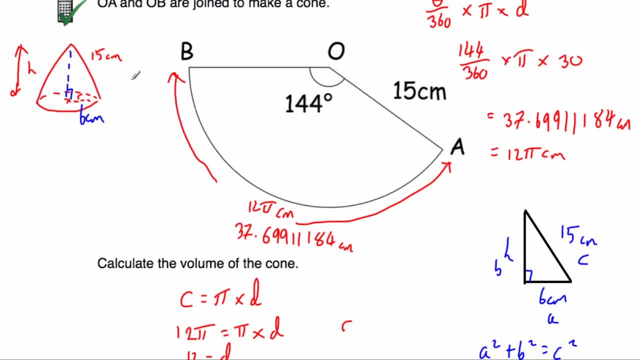 the radius of the cone is equal to 6. we've got the height of the cone, which is equal to. the height is equal to 13.74772708. now we can just work out the volume of the cone by using the formula. volume equals a third pi r squared h. so we're going to do third times pi. 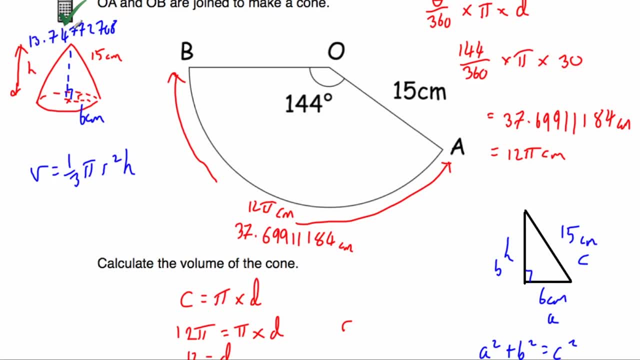 times 3 root 21 or 13.74772708 centimeters. so we've got: the radius of the cone is equal to 6 squared times by 6 squared times by 13.74772708, and when we do that we'll get the volume of the.